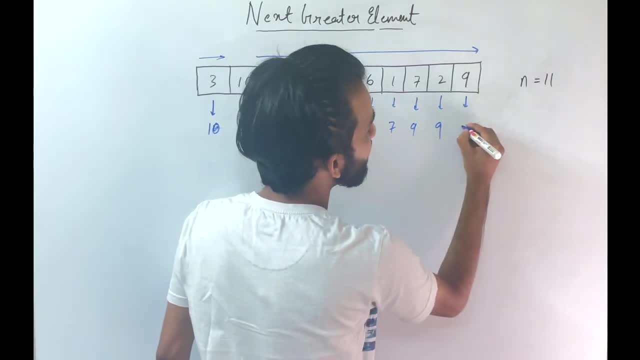 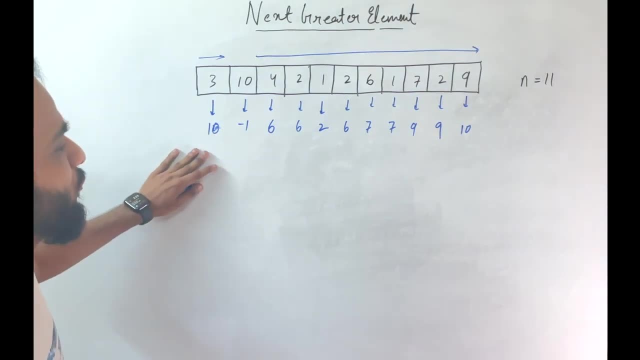 no, it's 10. the next greater of 9: yes, so for 9, the next greater is 10. so this is how the next greater element will look like. so you have to just print, or you have to return me this ng array. yes, you have to return me this ng array. next greater element array. now let's uh, first keep aside a very 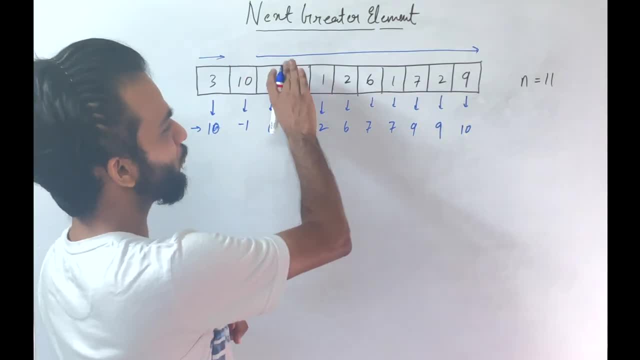 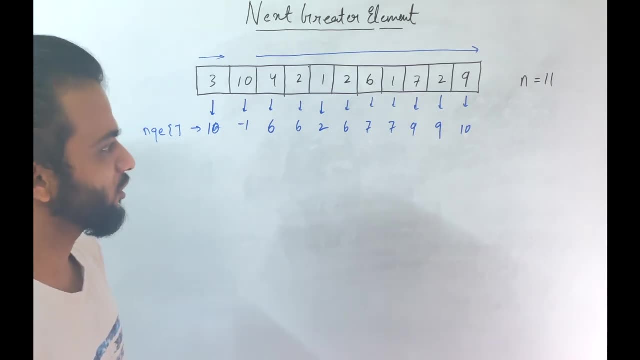 like this is a circular array kind of a problem. right, you have to. if you don't find it on the right, you have to look across from here as a circular array kind of problem. first let's try to solve the easier variant of this problem. what is the easier variant of this problem? 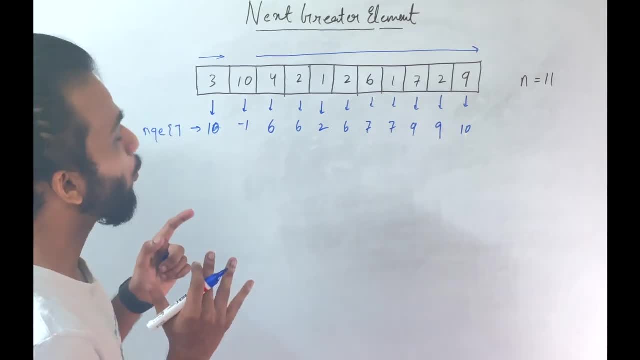 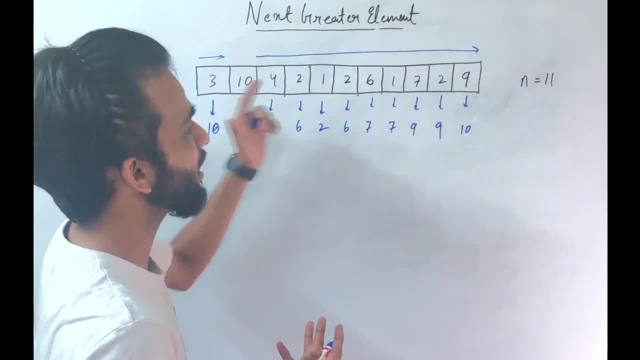 it's nothing, but i'll try to figure out which is yes, which is the on the right. i'll just try to, on the right now what i mean by i'll be figuring out on the right for 9. on the right, that doesn't exist any. once i'll. 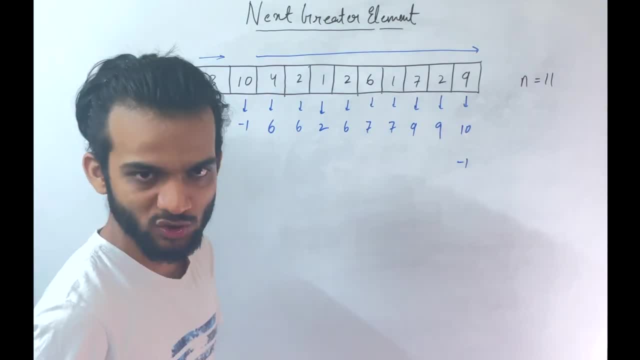 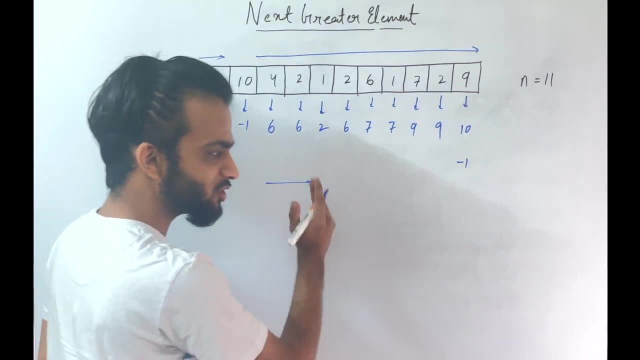 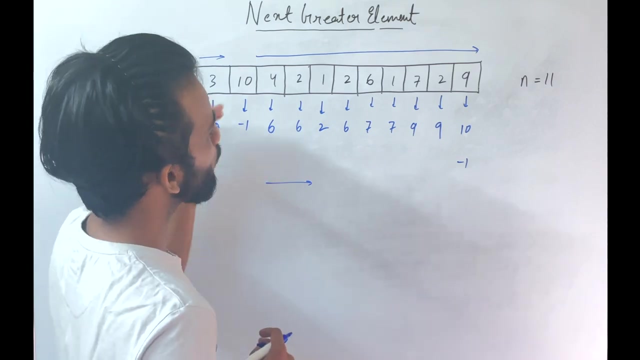 print a minus 1. that means i'll not be considering the circular array question as of now. the first variant that i'll be solving will just look across right. no circular one will just be looking across right and we will try to solve that problem. and after that- yes, after that- we will try to solve. 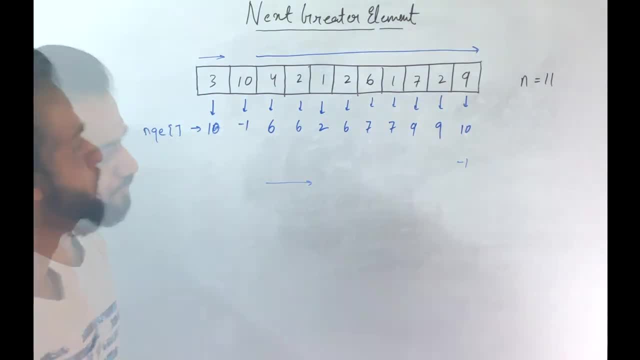 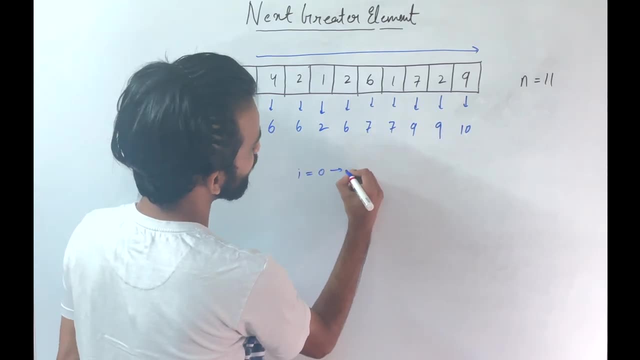 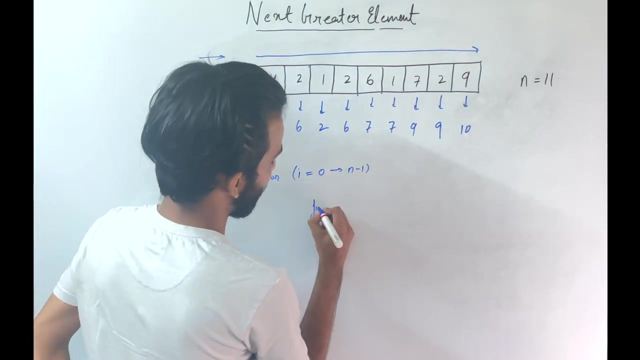 this circular variant because it will be just a minor change. so what will be the brute force? can root force will be nothing. but for every element from zero to n minus one, yes, for every element from zero to n minus one- i can definitely look on the right, and that right will be starting from j. 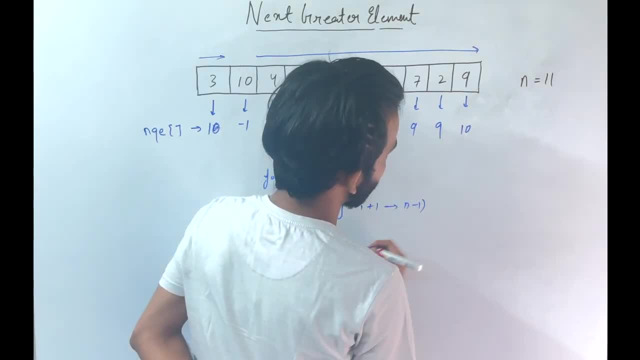 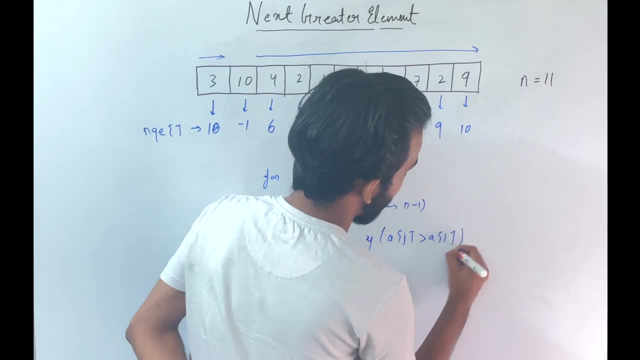 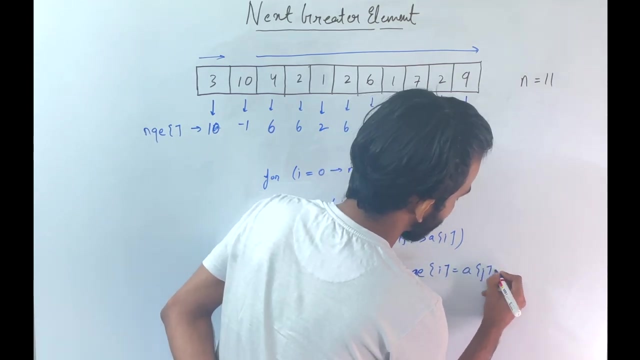 equal to i plus one, and i'll go on till n minus one. and whichever- yes, and whichever is a of j is greater than a of i, i can say that guy will be the next greater element of i, and i can put it. and once i've got the next great element, i can put a break statement and i'll break out. 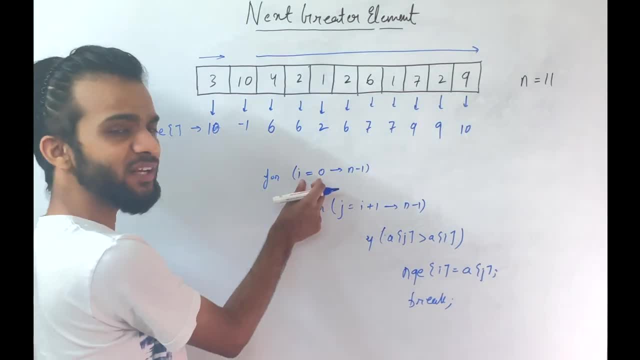 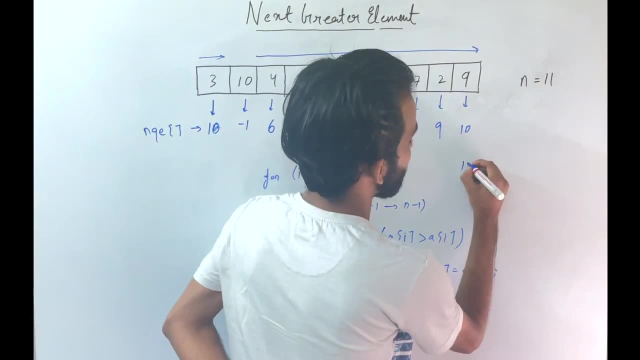 so this is how the brute force will look like. for every element, i look on the right and i'll figure out which is the next greater element. but imagine for an array like this: 10, 6, 7, 5, 3, 1- you will never. 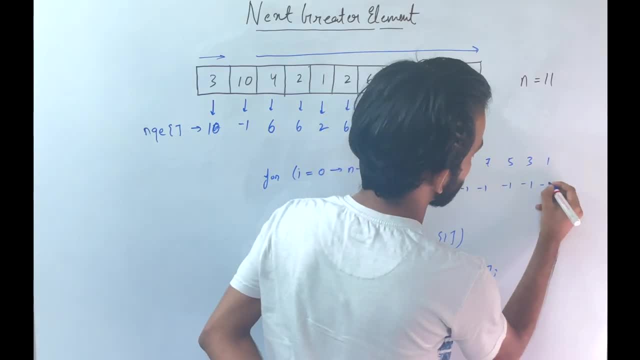 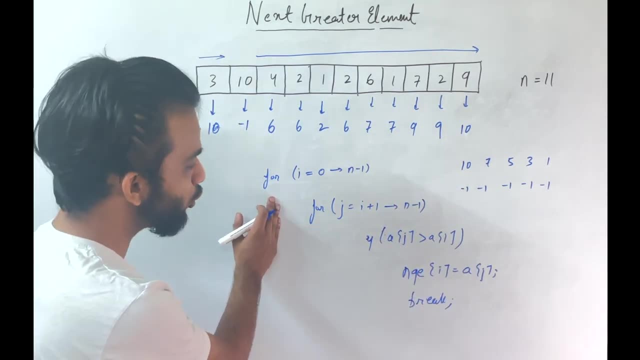 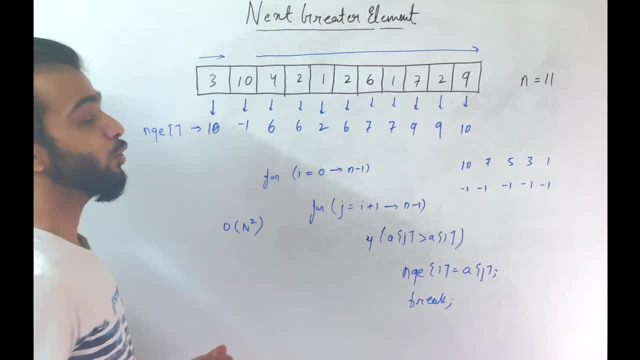 completely, and this is also gonna run till n minus 1 because i don't find any next great element. so the time complexity of the naive solution that you're gonna tell to the interviewer will be bigo of n square and obviously the interviewer will not be happy with this and he'll ask you. 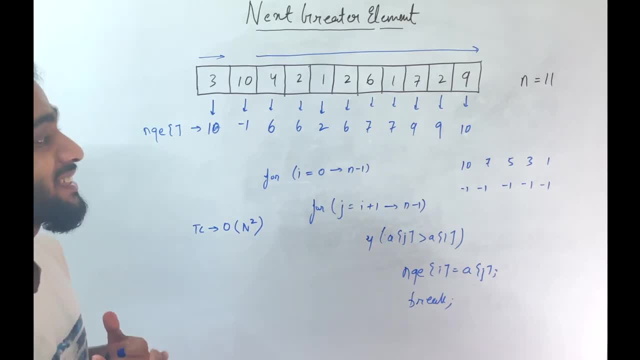 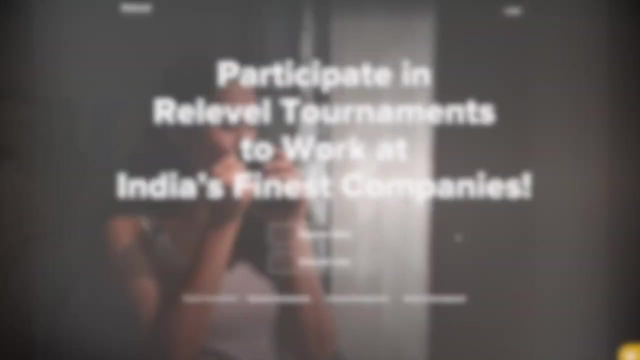 to optimize this. that is when we will be using stack. now, why stack and what is the intuition? you're gonna discuss everything, but first i'll tell you the algorithm and then i'll tell you the intuition behind that algorithm. so let's first understand the algorithm. so, before moving to the 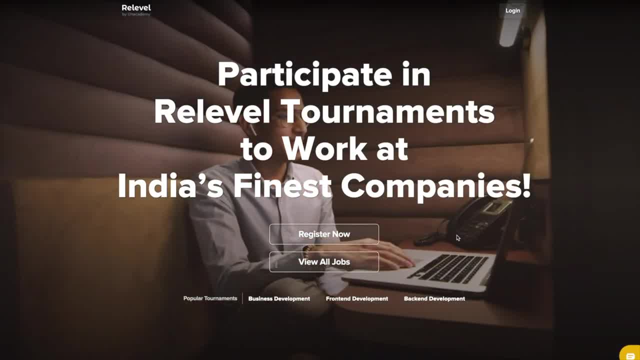 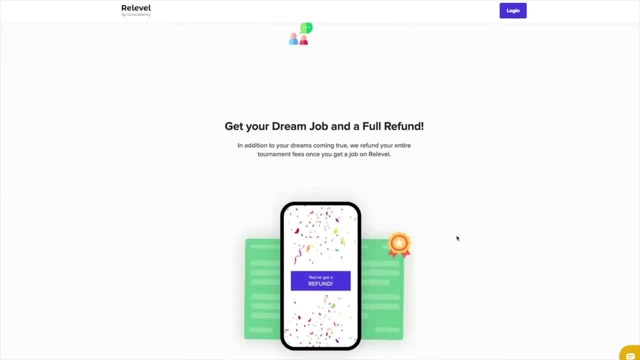 efficient solution. let me talk about the sponsor of this video. this video is sponsored by reliable, which is backed up by an academy. now, this is india's first hiring tournament platform where you can participate and you can get a chance to work with india's finest startups. so how this works is. 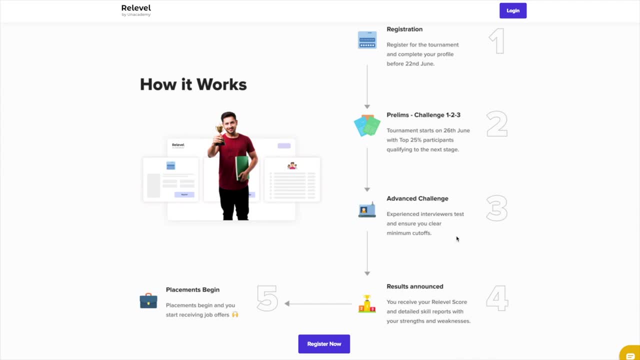 you have to register in the tournament and you have to participate. let's say you're in the top 25 of all the participants, you get a chance to interview at all these india's top startups and if you clear the interviews, you will be handed off with handsome salaried job offers. now you must 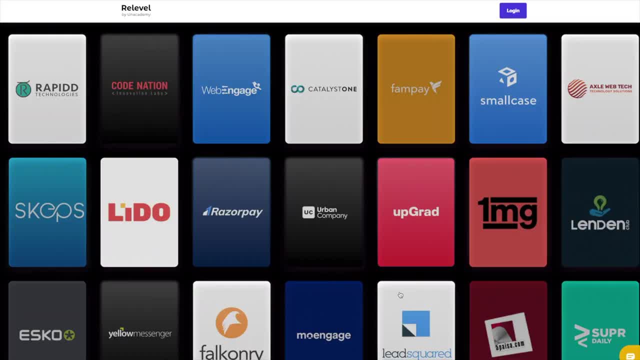 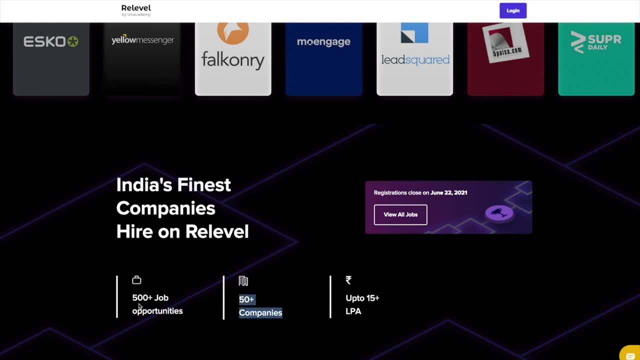 be thinking which startups, so reliable, has partnered with companies like razor pay urban company, upgrade 1mg, yellow messenger. now there are in total of 50 plus companies with 500 job opportunities. basically 8 to 10 openings per company they do have. and what is the ctc offered? 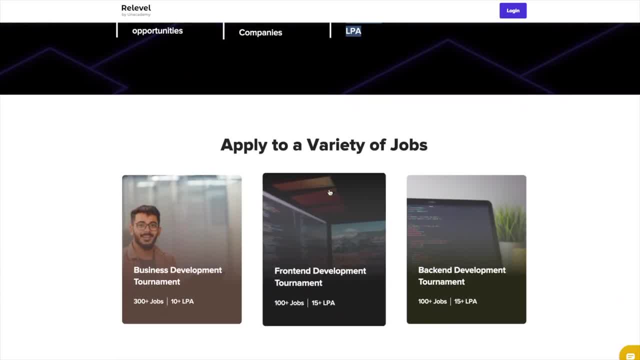 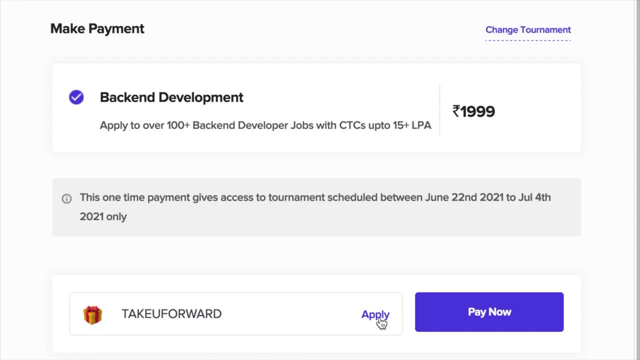 20 lpa. now, what kind of jobs can you apply for? you can apply for business development, you can apply for front-end development, you can apply for back-end development. now, the participation in the tournament will just cost you one triple nine and if you apply the coupon code, take it. 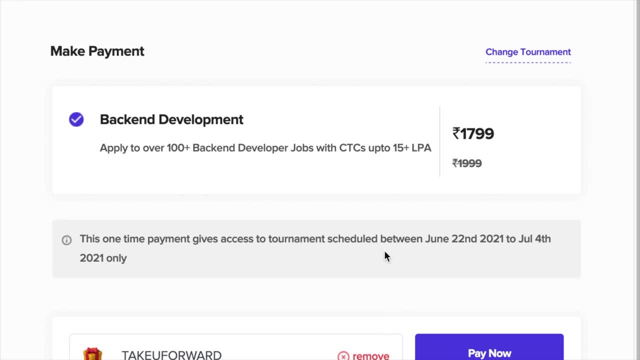 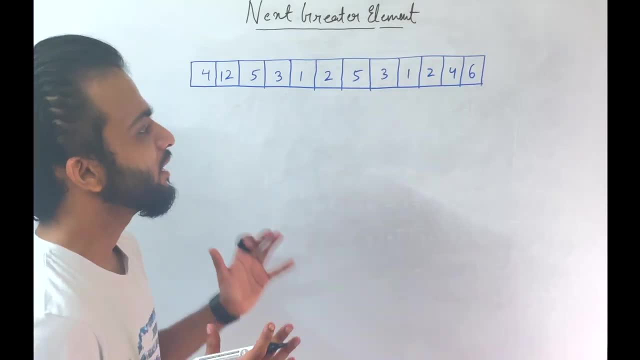 forward. it's gonna cost you one, seven, nine, nine, and the last date to register is 22nd june. so guys, go check it out and don't miss this opportunity. so the efficient solution will be using stack. so what you'll do is we will define a stack data structure, which will be an empty one. 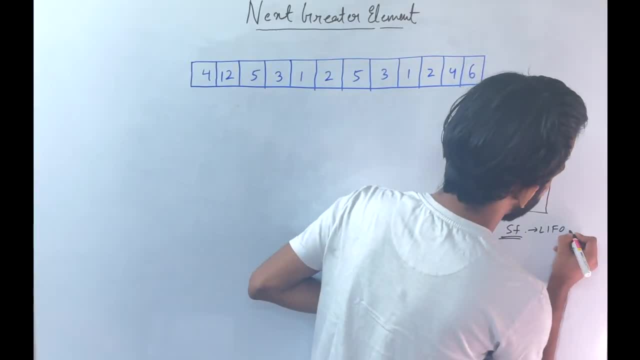 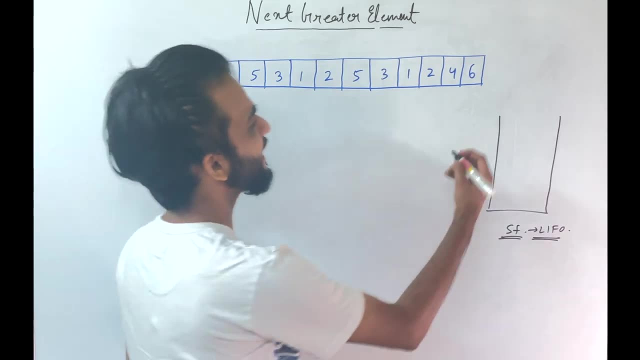 structure that is nothing but a last in, first out data structure. i've already made some videos on this. you can definitely watch them out if you don't know what is the stack. so what we will do is we will start iterating from the last element. the last element is nothing but six, and we will 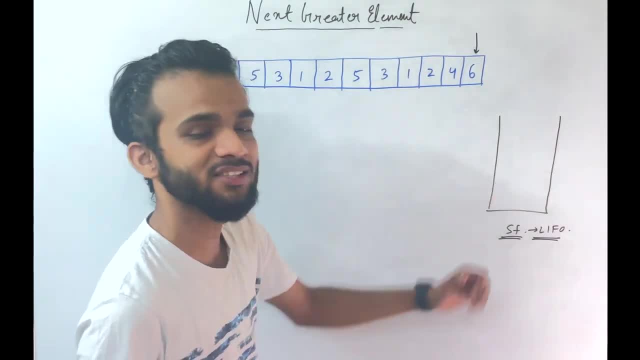 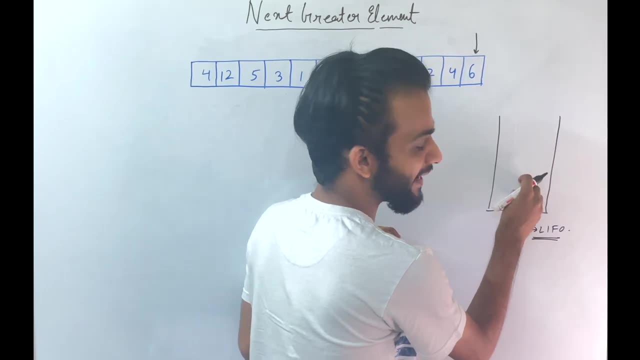 see if there are any elements lesser than six on the stack. i see that there are no elements lesser than six on the stack, so what i'll do is i will see if there are any elements on the stack. i see no, there is not a greater element. also, 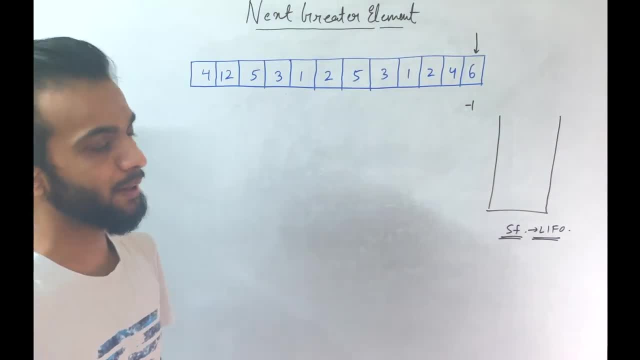 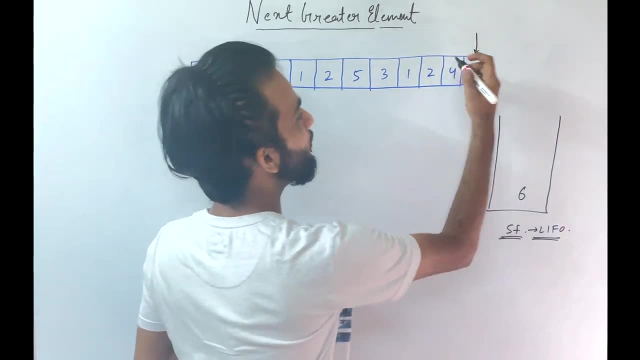 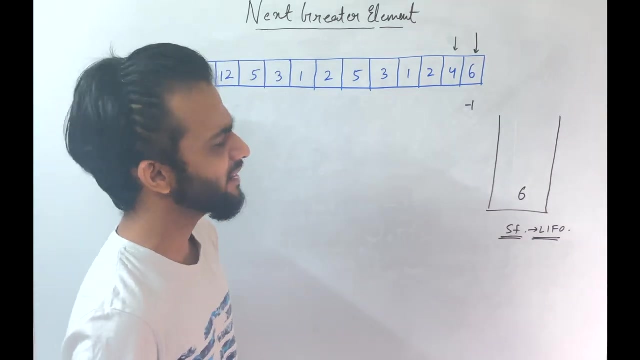 so i will take minus one and i'll put it over here. okay, done. once i've done that, i'll take this six and i'll insert that into my stack. right after that, i'll move my pointer to the next element four. four now checks if there are lesser elements and it finds that there are no lesser elements. 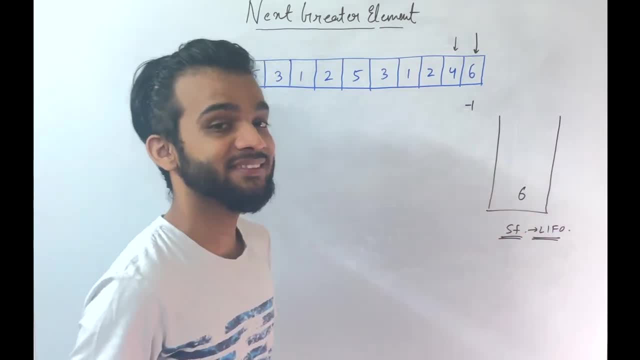 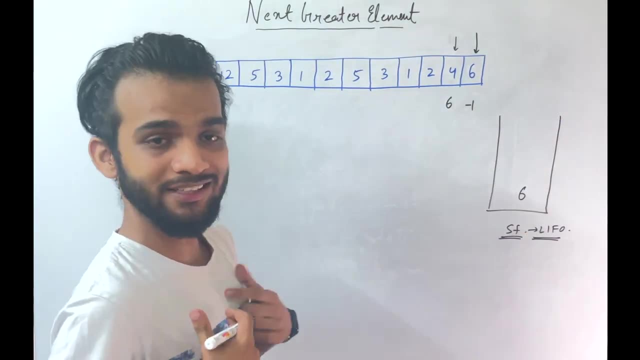 so now four says who is the topmost element in the stack. it sees six. so he'll take six and say, okay, since there are no lesser elements on the stack. well, i'll say if that lose six, so he 행 gets three, because he see is five, it gets six. 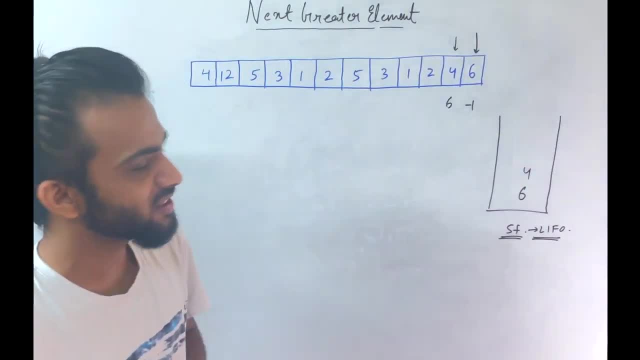 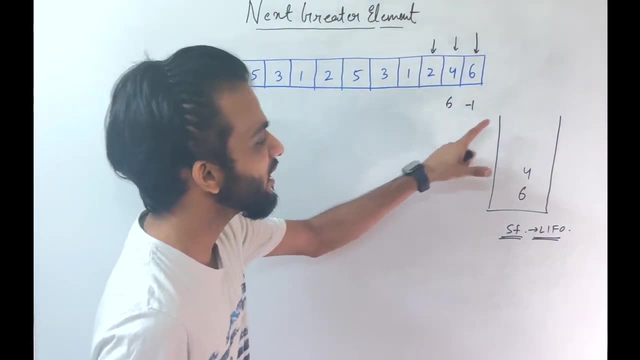 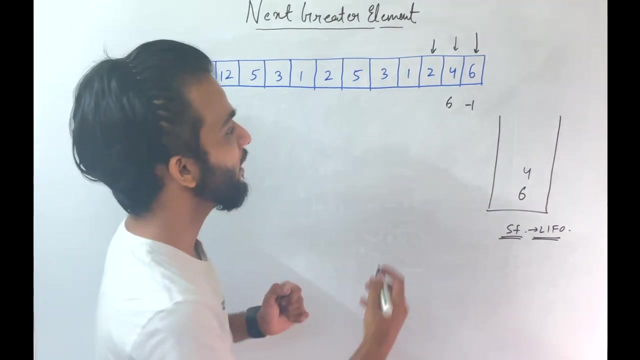 so what i'll do is i'll take the top most guy six and that will be my next creator element. after that he takes this four and inserts it into the stack. right after that it goes to the next element, that is two. again two checks if there are smaller elements on the stack. no, there are no. 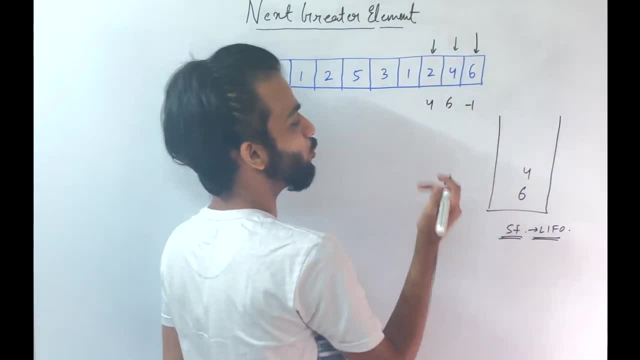 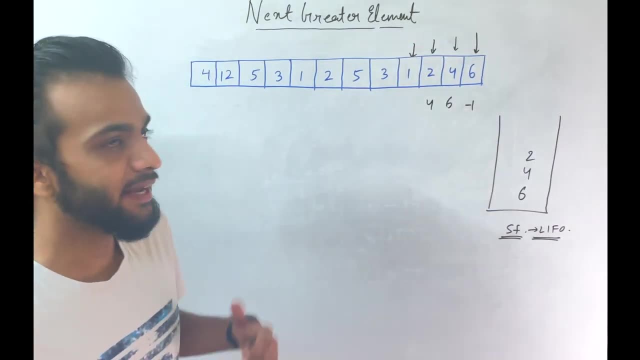 small elements. so two will take the top most element, that is four, and he will say: four is my into the stack. Right after that you will go to this one guy and again one will do the same thing. Are there elements lesser than one on the stack? I see that there. 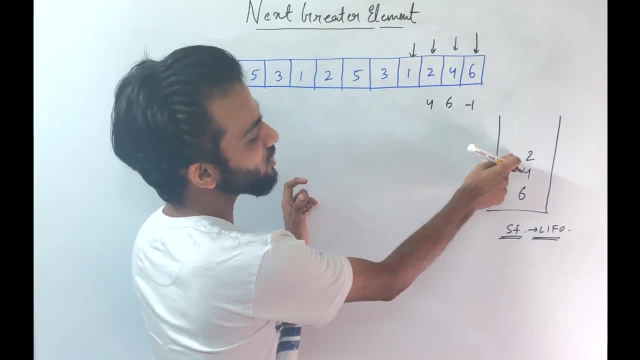 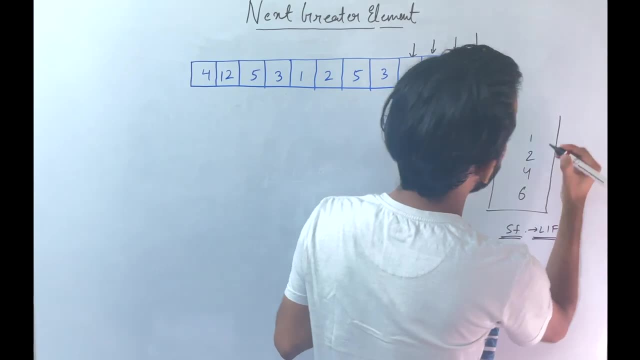 are no elements. So what it will do is it will take the topmost guy and say: it is my next greater element. Fine, After that you will take that one and it will insert it into the stack. If you carefully observe, a pattern has been made. The 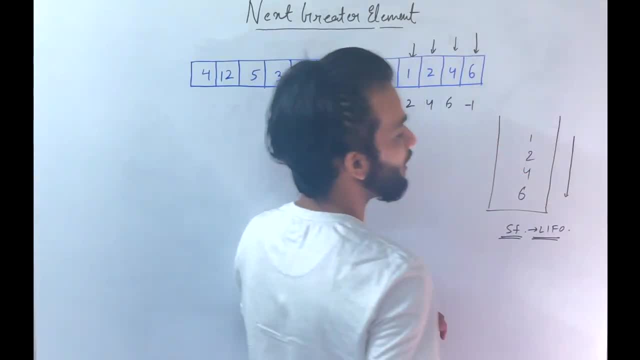 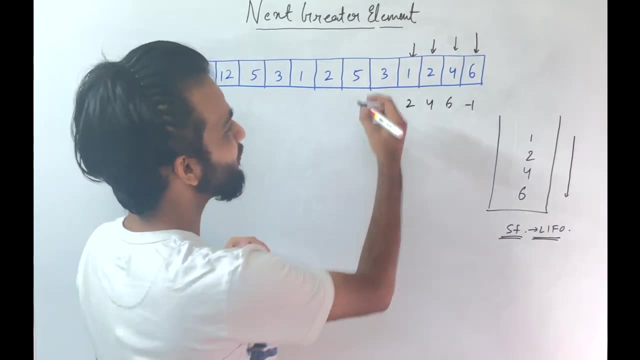 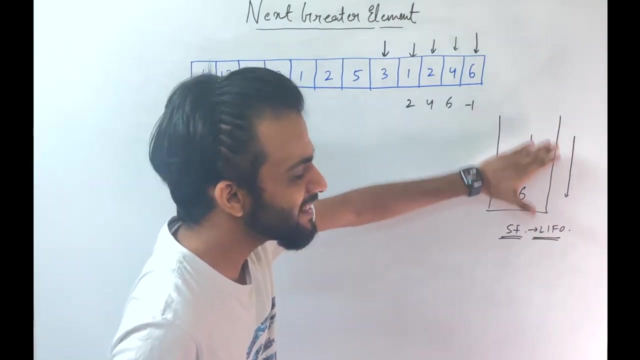 stack is containing elements from top to bottom in an increasing order. Yes, in an increasing order. You see that pattern forming right. So after that, when you come to three, When you come to three, If you want the next greater element in this increasing order, you need to remove all the smaller elements than three. So, 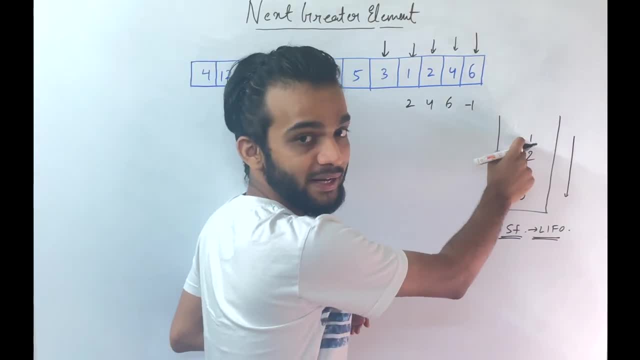 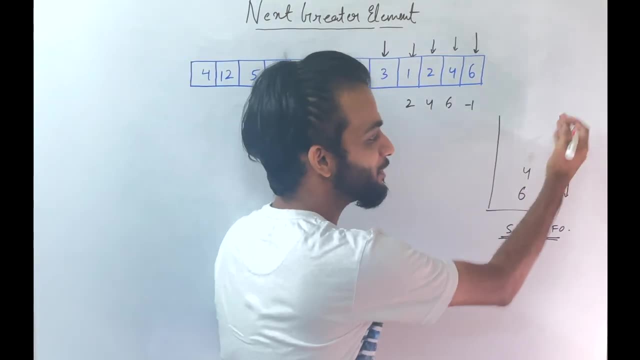 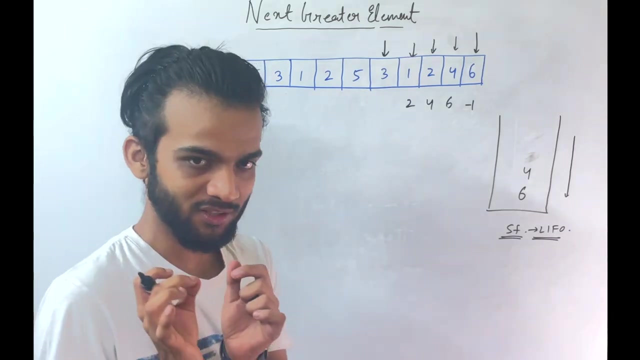 first three compares it with the top. It is small: Remove. Then three gets compared with two: Remove. Since it was an increasing order, you made sure that all these small elements than three were removed right after that. Right after that, Three sees which is in next top element, that's four, which is greater than three. 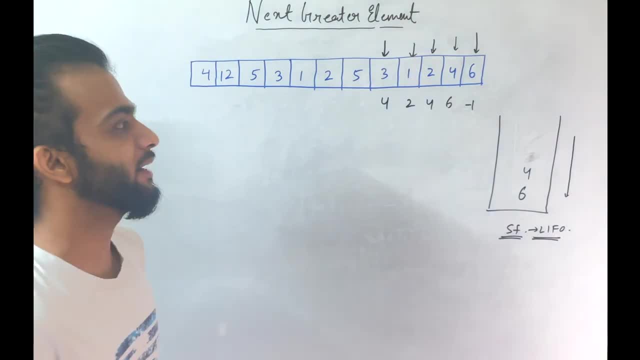 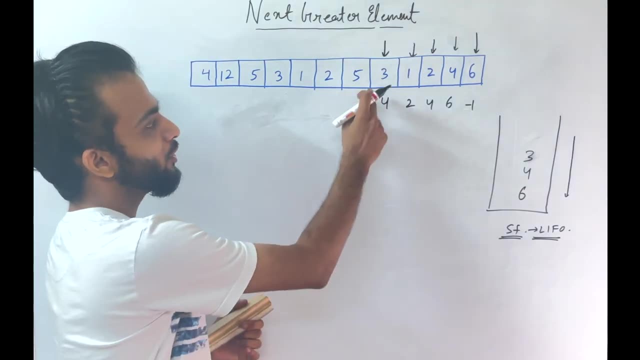 Hence it becomes the next great element, and this three will get into the stack. Now you might be thinking: hey, Striver, you wrote three, but you removed one, two. This 1, 2 is removed, but it might be an answer for someone else. 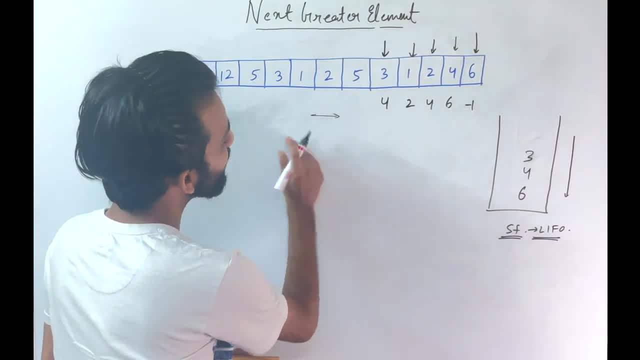 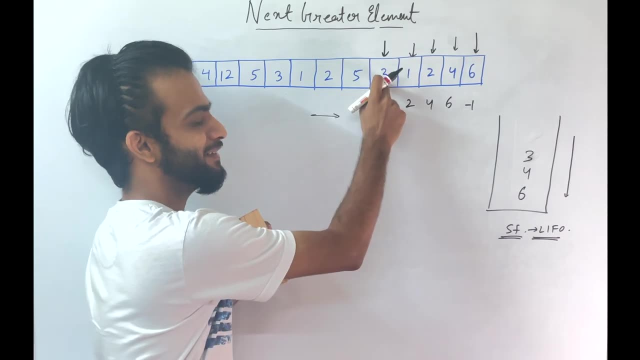 No, yaar, how can it be an answer? Just imagine, if you are looking from this angle on the right, if 3 comes before 1 and 2.. So if 3 is coming before 1 and 2, 3 will obviously be the next greater of anyone on the left. 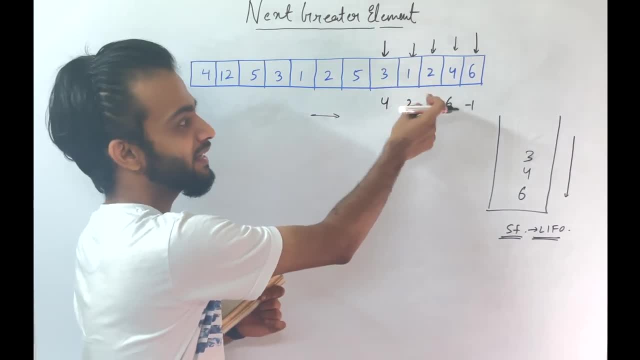 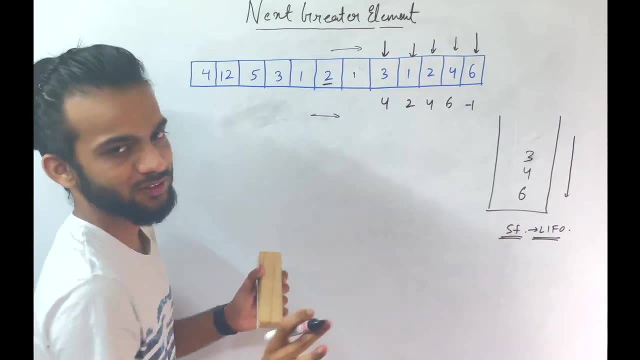 1 and 2 can never be, because 3 is already greater than 1 and 2, right For this 2, if you look on the right, just imagine this was something like 1, just imagine Then for this 2, this 1 and 2 can never be the next greater element. 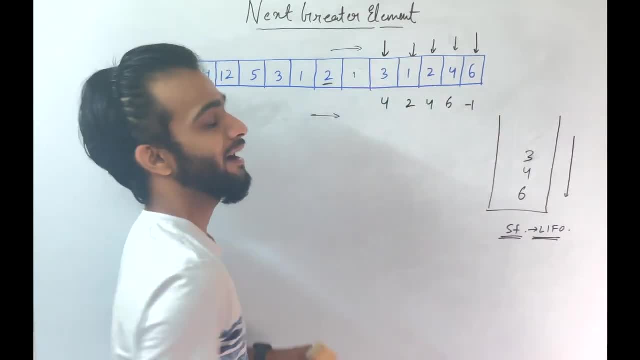 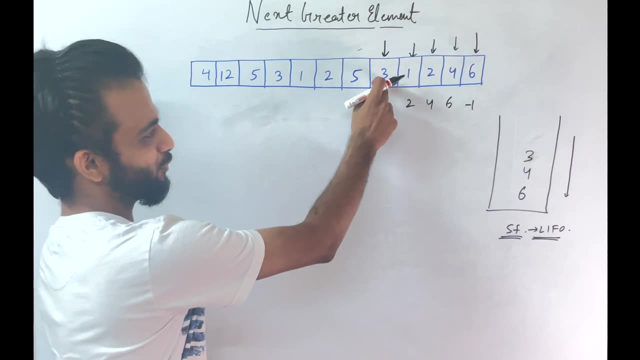 This, 3 will only be. That's why 1, 2 have no significance and you can definitely remove that. So I hope you have understood the intuition of removing 1, 2, because if 3 is there, 1, 2 can never be the next greater element. 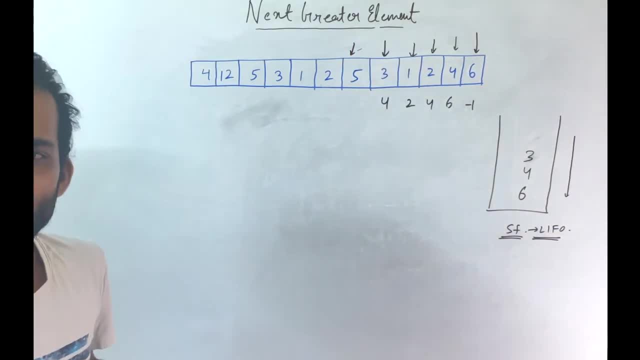 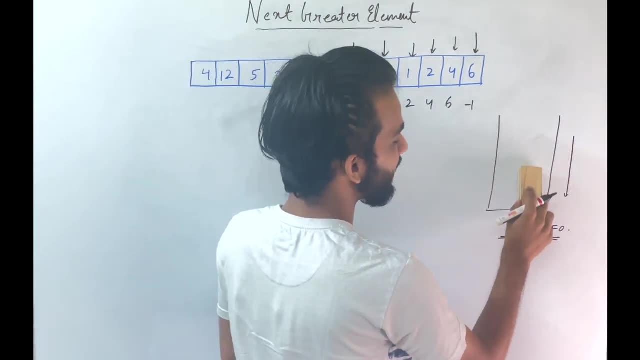 Okay, so 3 has been inserted. Next come to 5.. Again, do the same thing. It's following an increasing 10.. So remove all these smaller elements. 3 will get removed, Then 4 will get removed. 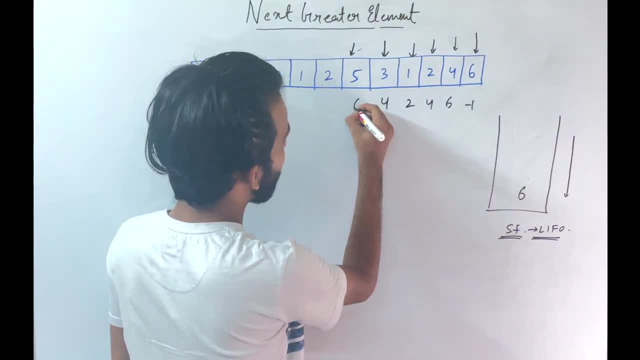 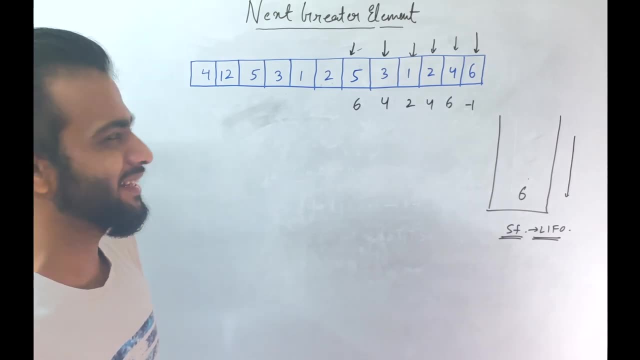 Right after that, whichever is the element that will become my next greater element, Again makes sense. I removed 3.. 1 and 2 I previously removed because they can never be the next greater element. So as of now I have 5's next greater as 6.. 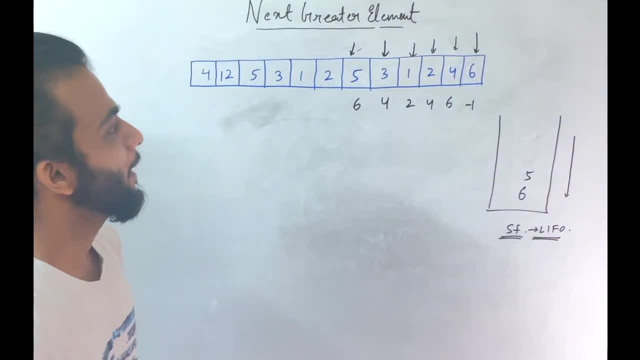 Take 5 and insert that into your stack Done. Come to the next graph 2.. 2 C's are the smaller elements And it sees that there are no smaller elements. So what he will do is whatever is it at the top. he will take that and he'll say that: 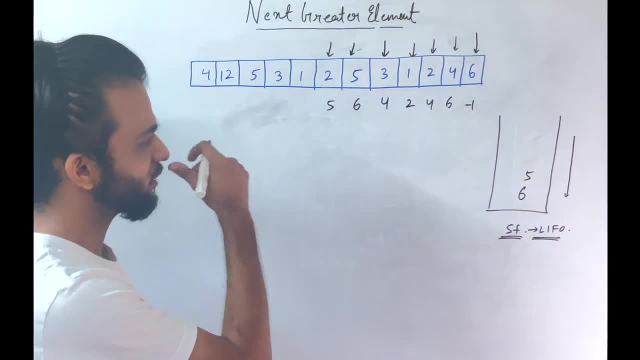 okay, this is my next greater element, So I've taken that Right. after that, 2 will get back into the stack. Now let's move. I come across 1.. 1 sees that there are no smaller elements. 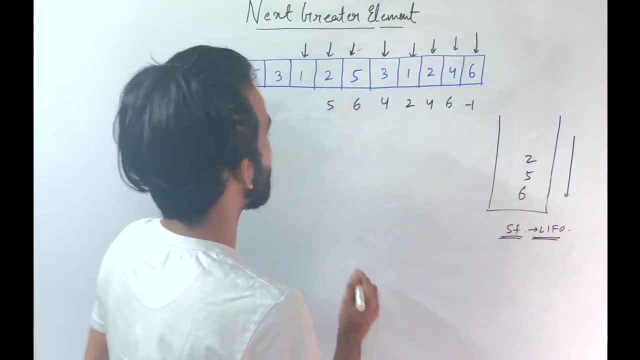 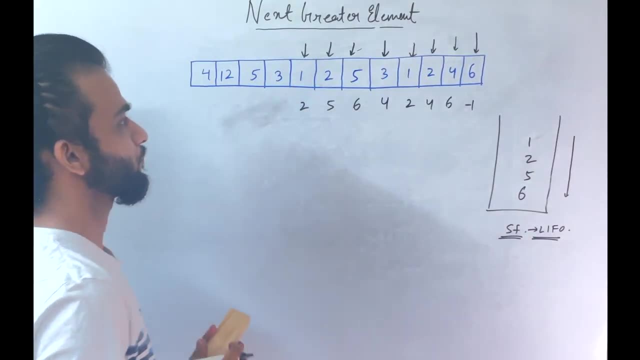 Hence, it doesn't remove anyone, But 1 sees the top guy to be 2.. Hence, that will become its next greater And it'll take this 1.. So I removed that over here. Right after that you will move to something which is 3.. 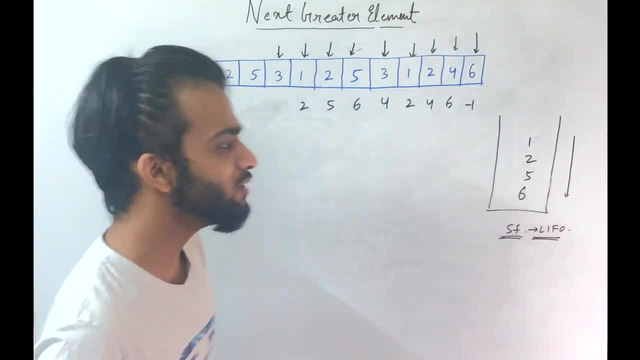 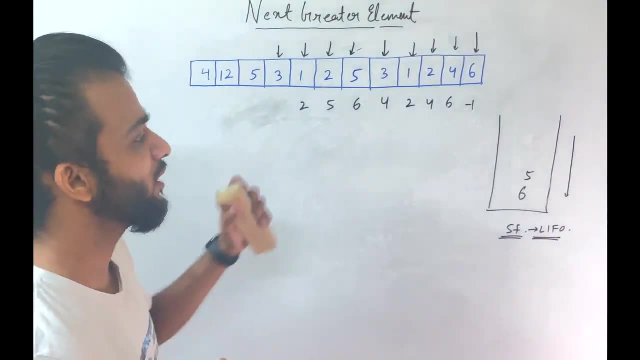 For this 3, again, you know it's appalling in increasing fashion. Kindly remove all these smaller elements. So 1 will be removed. 2 will be removed. So I've removed all these smaller elements. Now for 3,, which is the next greater element. 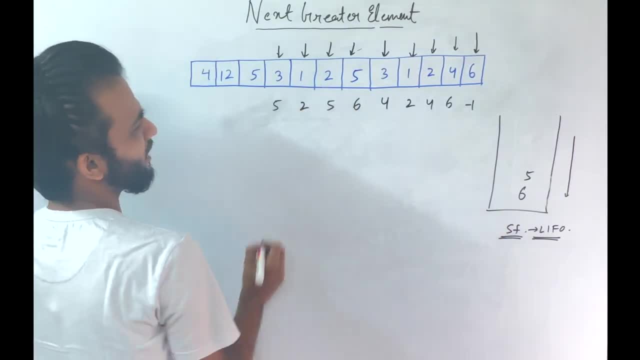 5. So again you write 5.. Again very obvious, because for 3,, 1 and 2 will never be of any use. So 3's next greater is 5.. Take this: 3. Insert it. 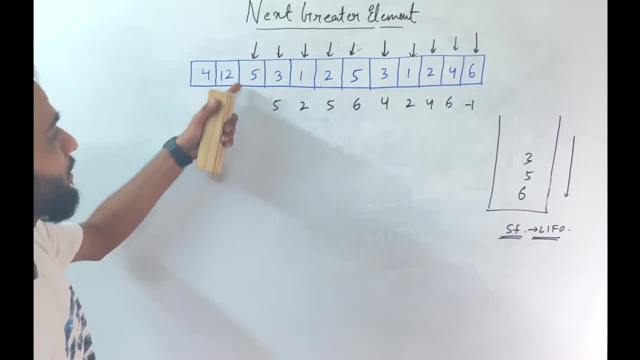 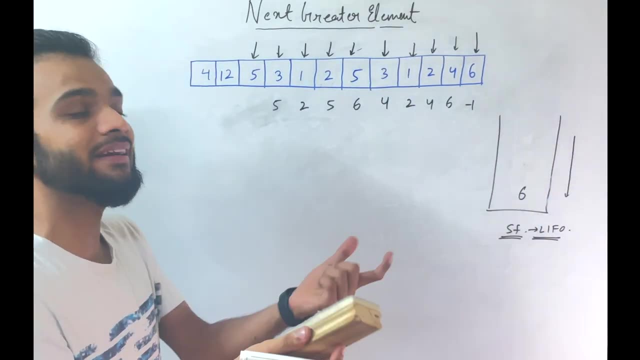 Right after that you come across 2, something as 5.. 5 will remove 3 as well as 5, because it wants the next greater element. So 5, 6 is the next greater element. So you'll take that. 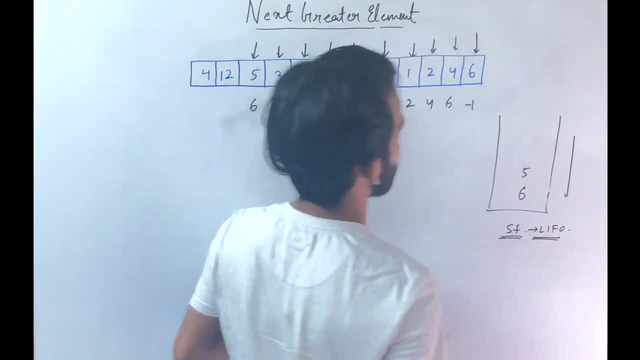 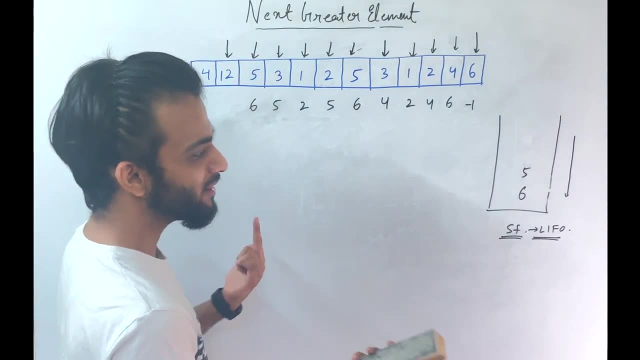 Now take this 5 and now again insert that. So this is how the stack will be. now Let's move to 12.. What 12 will do is 12 will remove all these smaller elements. 5 is removed. 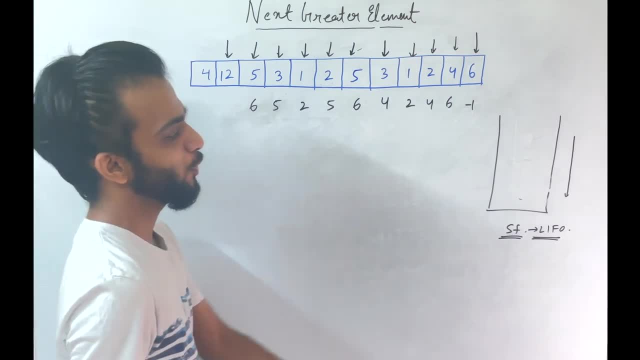 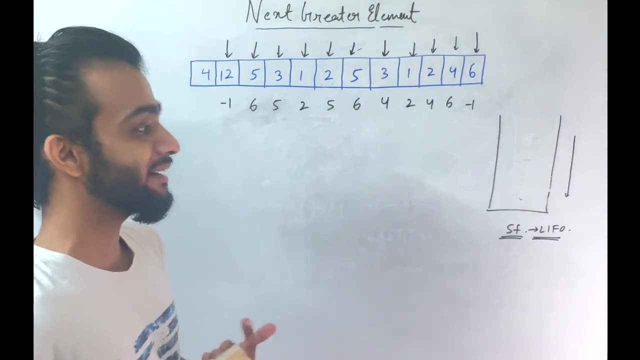 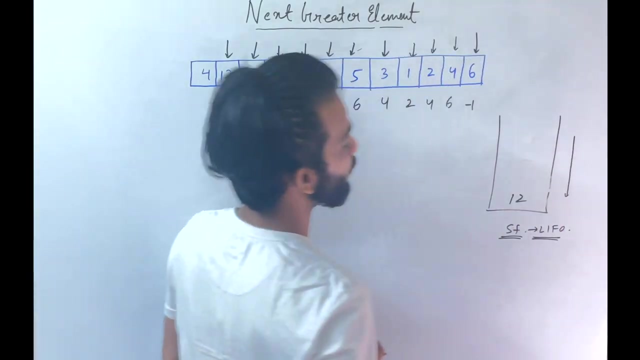 6 is removed. Apparently, 12 removed all the elements from the stack. Hence I can say that 12 doesn't have any greater element. That is why stack is empty. I can say minus 1.. And I'll take this 12 and I'll insert that into my stack. 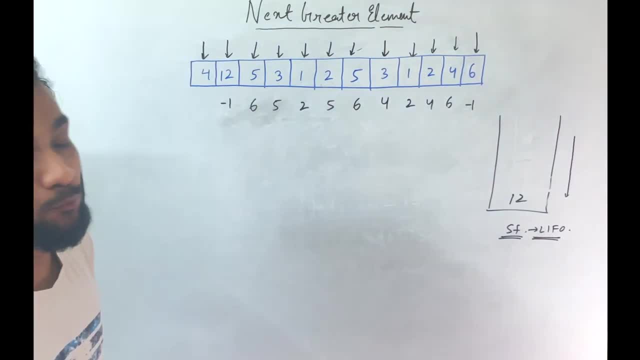 Right after that I'll come to 4.. Yes, right after that I'll come to 4.. When I come to 4, I will again look if there are smaller elements. I don't find any, So I'll take this 12 and I'll say: 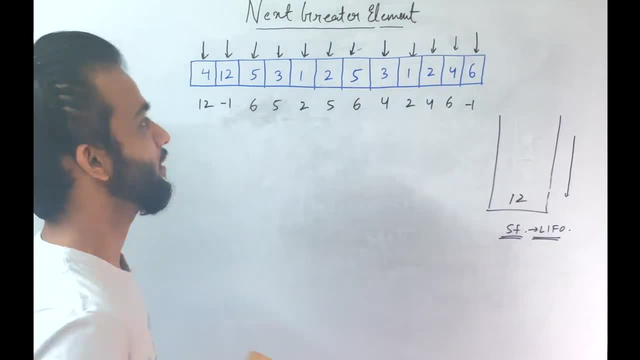 that's your next greater element, And once I've said that, my pointer will move beyond. Hence I've traversed from the last to the first and my next greater element array is ready. That's going to be my answer, So I hope you've understood the intuition while I was explaining. 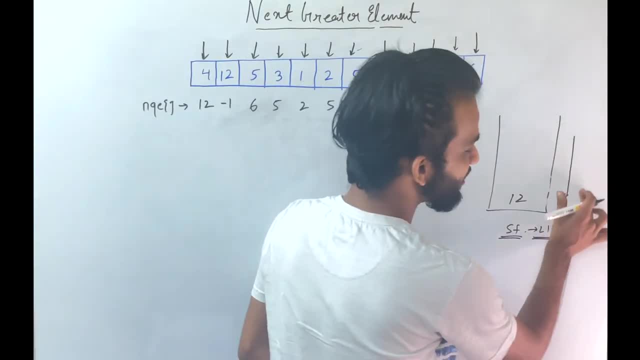 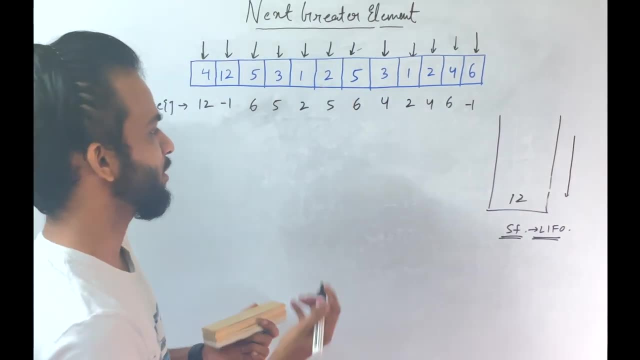 The intuition is very simple: I want to maintain an increasing order so that I can easily remove these smaller elements. right, Because the smaller elements do not have any sense, because if I'm looking on the right, if there is someone as 2x. 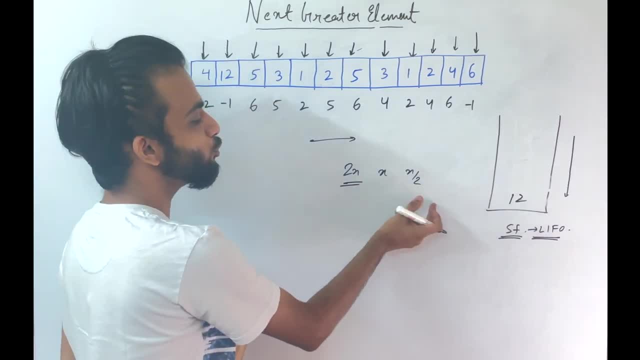 these x or x by 2 elements will be of no use, Because for someone who is x or this x, this 2x will be the next greater, not these guys, Because when he'll travel, he'll travel, he'll find 2x at first. 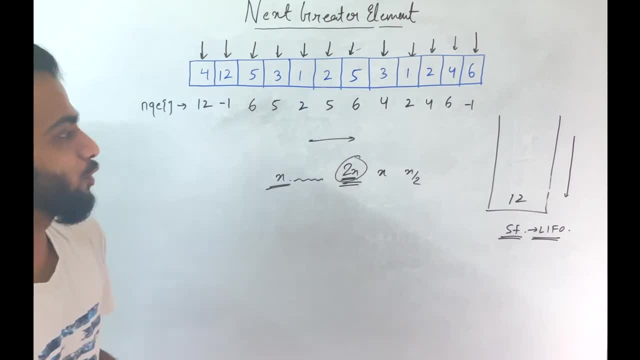 That's why removal of smaller elements is so important over here. So this is how the first variant of the problem can be solved. Now the original question. let's come back to the original question. The original question stated you have to also figure out the circular one. 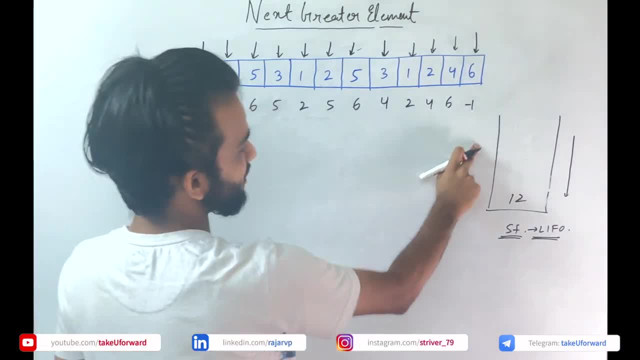 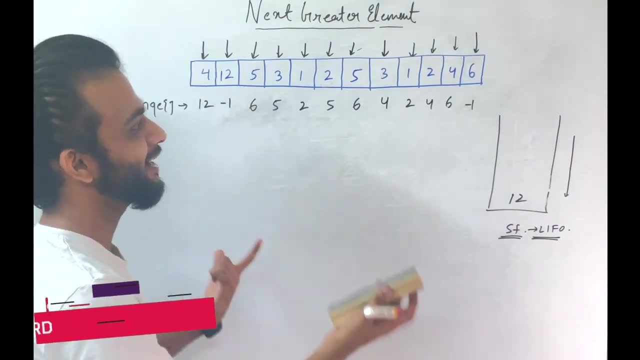 Like for 6, the answer will be 12.. Figure out the circular one. So let's take a smaller array and tell you how to convert this similar logic to the circular array. So this is the example for which we will be implementing the circular variant. 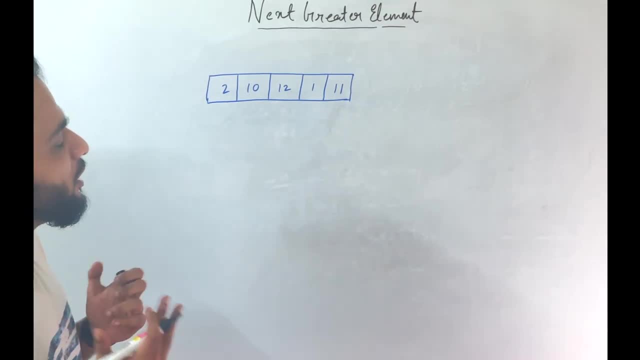 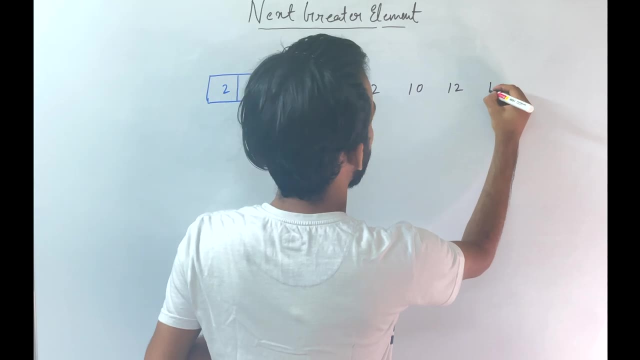 Now, in order to solve this circularly, what you will do is you will just copy paste the same portion once more, So that's going to be 2, 10, 12, 1, 11.. Once you have copy pasted it, 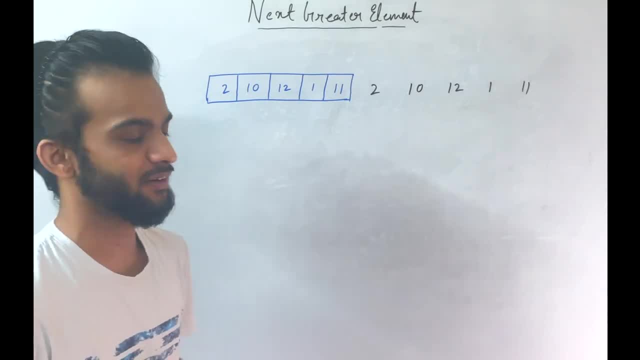 just solve it as you solved the first variant. Just solve it on the right side. So if I solve it on the right side for those two, look on the right- it comes as 10.. For this 10, look on the right. 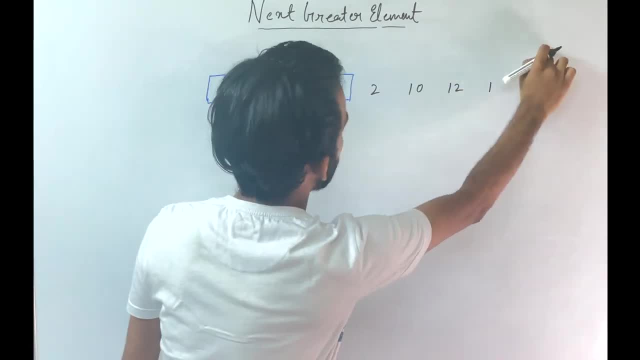 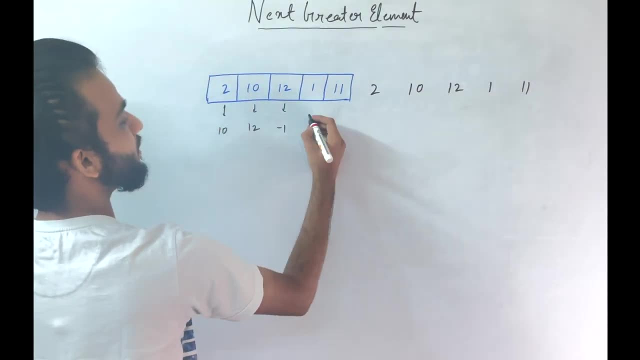 comes as 12.. For this 12, look on the right. what does that comes? No 1.. For this 1, look on the entire right. this comes as 11.. But for the 11,, when you look on the right. 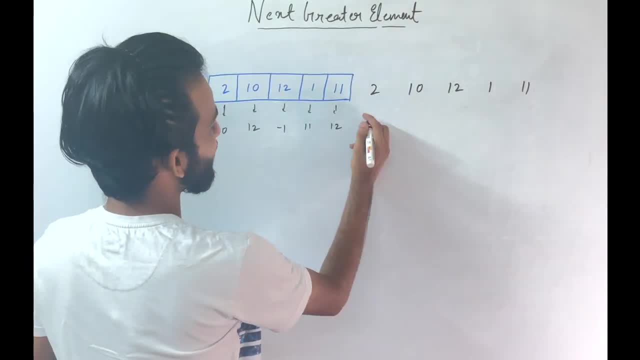 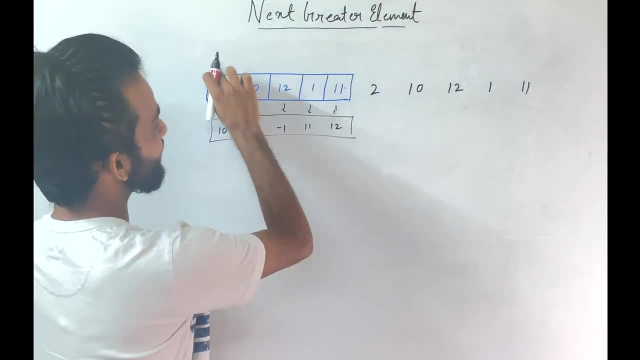 12 comes in. So you just need to figure out the answer for the first five elements. If you copy paste it twice automatically for 11, these portions will come at the front and you will be able to solve the problem using the logic that we implemented. 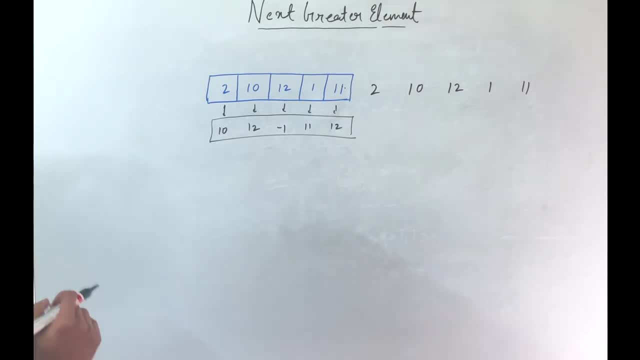 in the first variant of this problem. Now, how will we actually solve this problem? How will we actually implement this? Now, in order to implement circular array, you don't have to do anything. It's a very easy thing If I write the indexing. 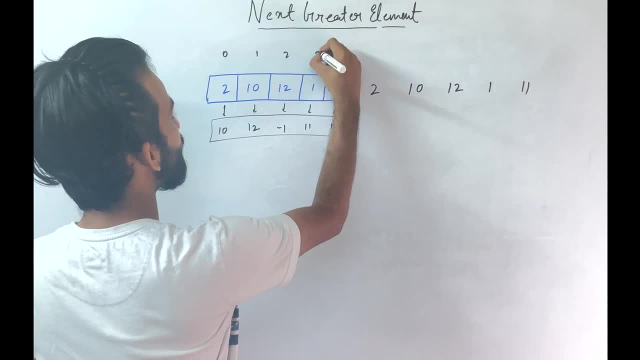 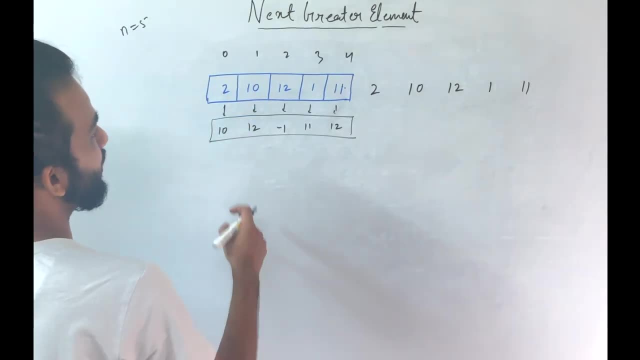 yes, if I write the indexing, it's a 0,, 1,, 2,, 3, 4.. That's for n equal to 5, the indexing is generally 0,, 1,, 2,, 3,. 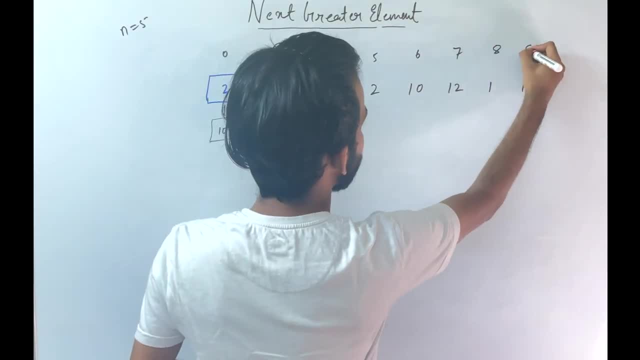 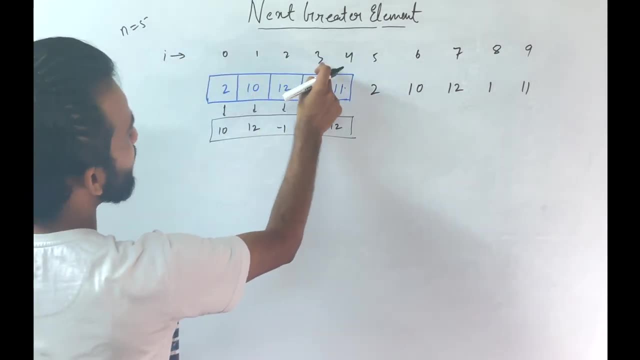 4. What you will do is: from 0,, 1,, 2,, 3,, 4, you will start having 5, 6,, 7,, 8, 9.. Just iterate: 0, 1,. 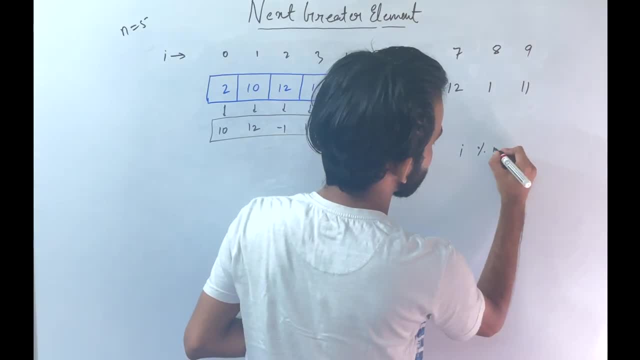 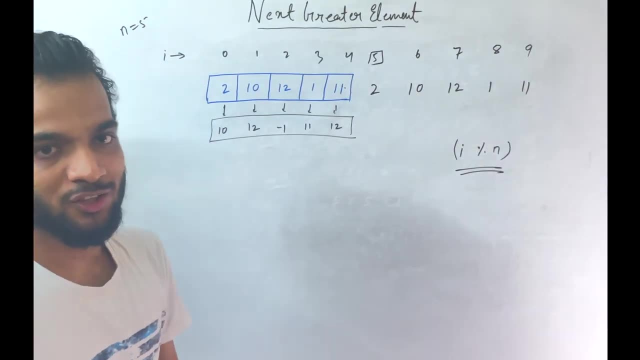 2,, 3,, 4,, 5,, 6,, 7,, 8, 9.. What you will do is this: i, if you do a modulo n, yes, if you do a modulo n, what will happen is: 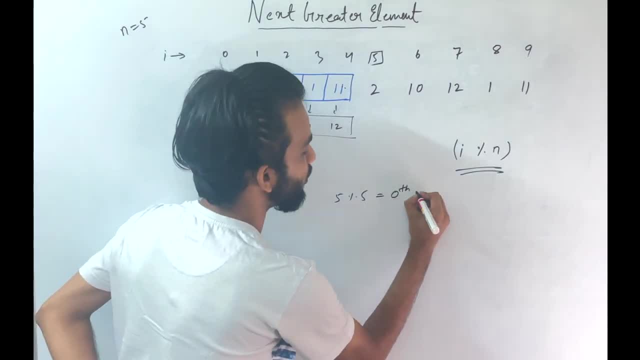 so let's imagine you are at the 5th index. So in order to get this 2, you will just have to do 5 modulo 5,, which is the 0th index. You will get the 0th index. 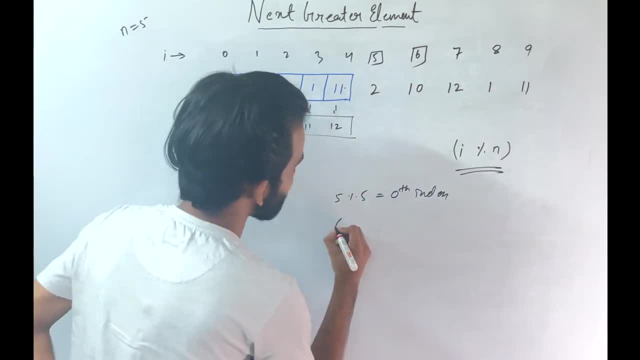 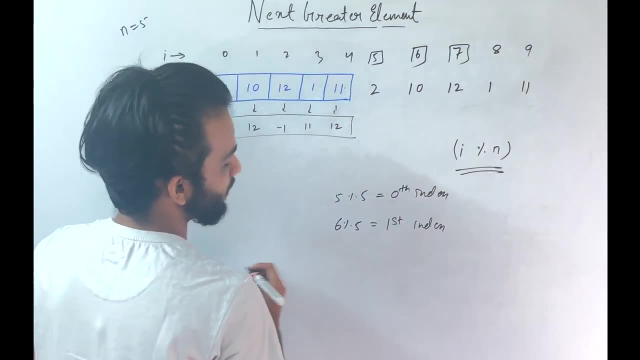 Now let's imagine you are at the 6th, So 6 modulo 5 will give you the 1st index. Next, imagine you are at the 7th, So 7 modulo 5 will give you the 2nd index. 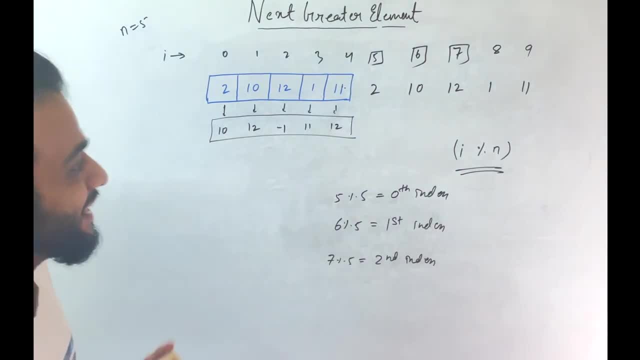 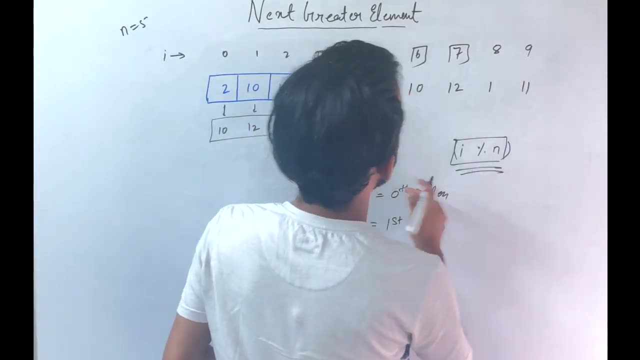 So it's an imaginary array that you are thinking. Yes, it's an imaginary array that you are thinking. You don't need to create this array because if you implement i modulo n, you will automatically get 2,, 10,. 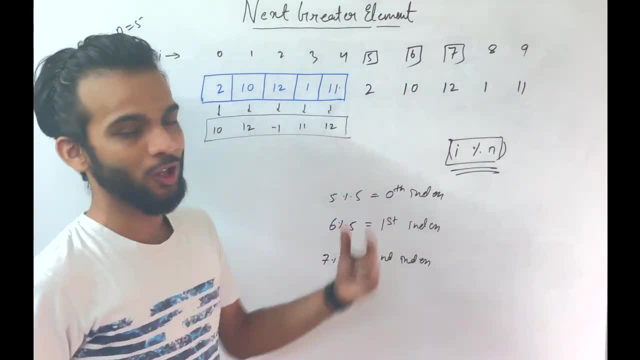 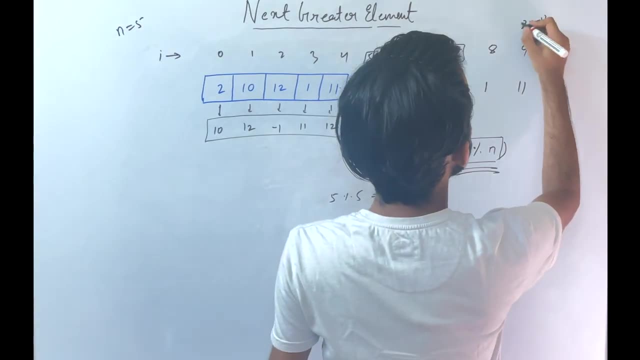 12, 1, 11.. You will automatically get all these guys, So it's very simple: From 0 to 2n minus 1 is the index where you have to iterate, And the logic will still stay as the first variant. 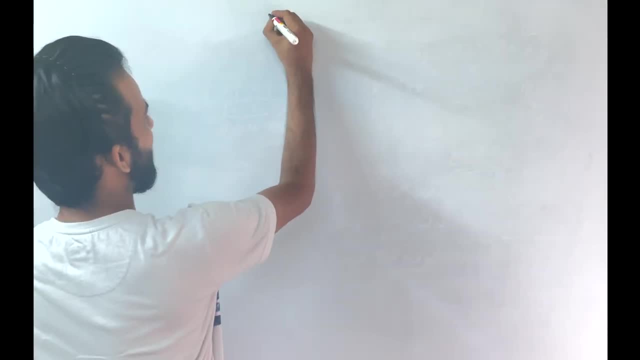 So let's try to write the code. So imagine I am looking for the answer in the NG array, So I have to declare an NG array of size n, correct? And I know one thing for sure: I will also require a stack. 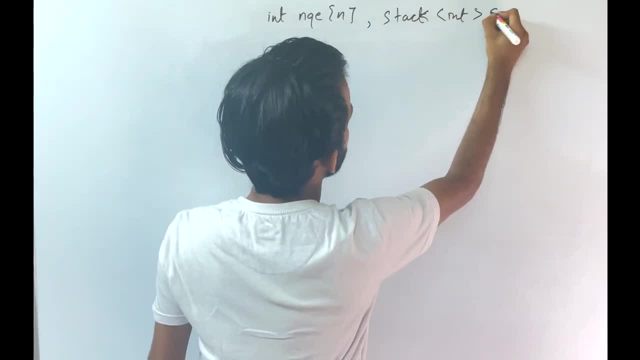 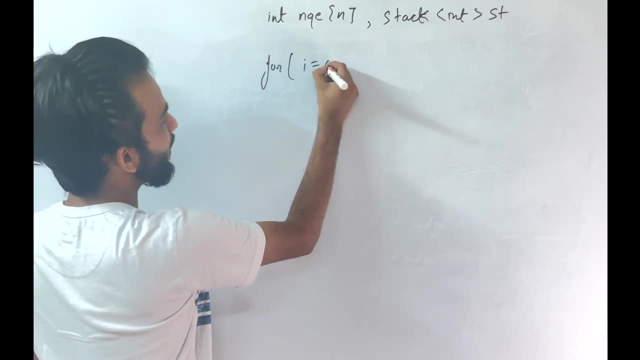 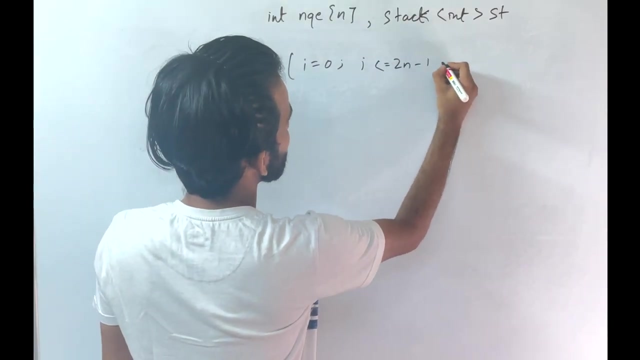 So definitely declare a stack of an integer, Some declaring these things, some declaring these couple of things- that will be required. One thing I know: my iteration will go from 0 to twice, So it's going to go till 2n minus 1.. 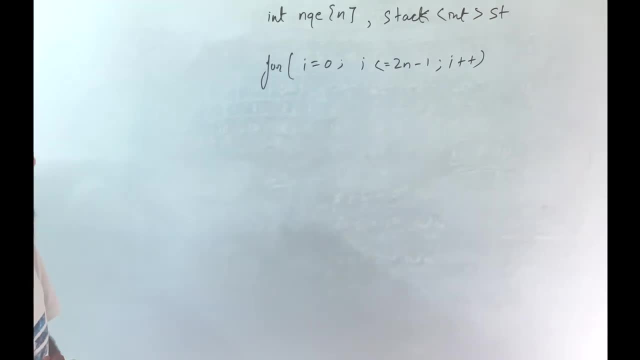 So why don't we go till 2n minus 1?? Now, what did we do at the first instance? First instance, we removed all these small elements of the stack. If you remember, the stack contains elements in the increasing fashion. 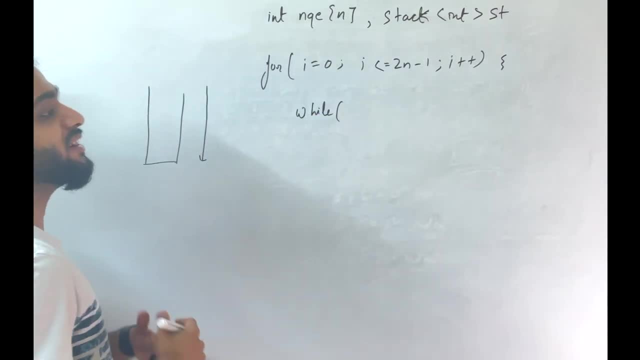 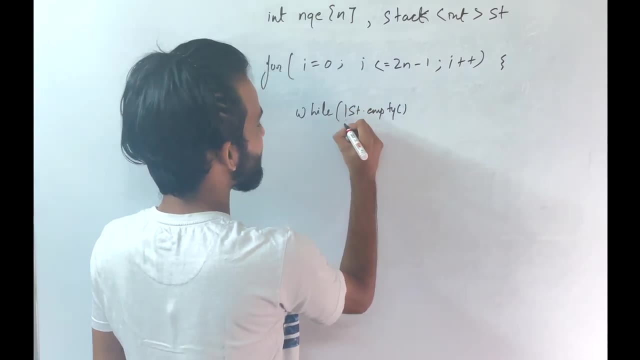 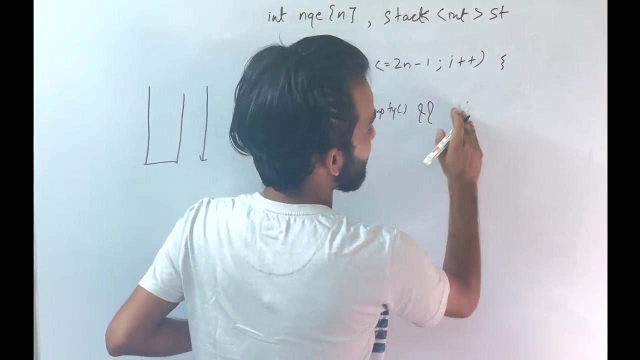 So what I'll do is I'll try to remove all these smaller elements. So if the stack is not empty, if the stack is not empty, then I will remove all the elements that are smaller than, yes, that are smaller than equal to a of i. 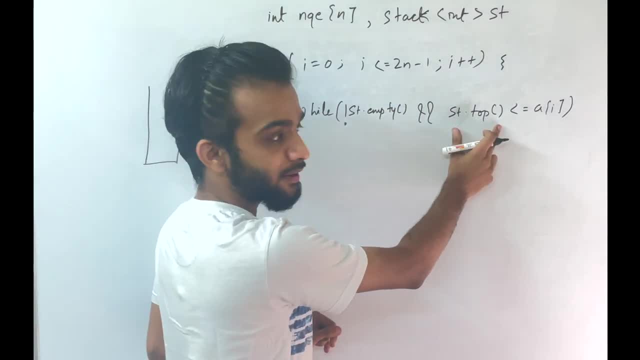 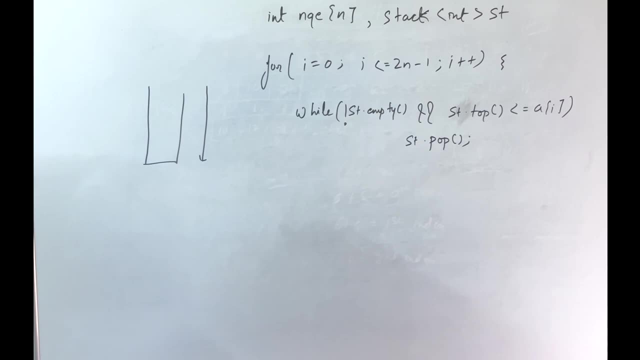 If the stack is non-empty and the topmost element is smaller than a of i, I will say: hey, why don't you remove yourself? So I'll remove all these smaller elements. Once all these smaller elements have been removed, 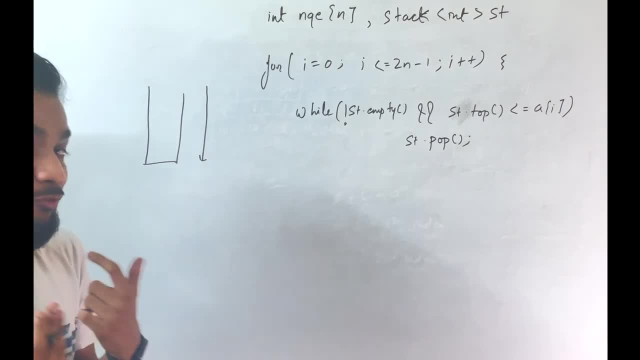 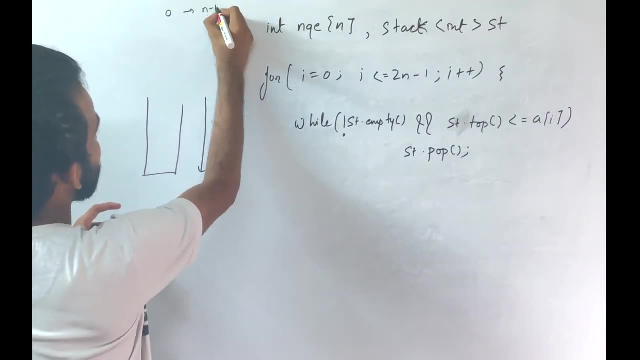 I need to assign. I need to get the topmost element, because that will be my nge. So I know one thing: I only required the indexes from 0 to n minus 1.. That is very much clear, because I've copied the array twice. 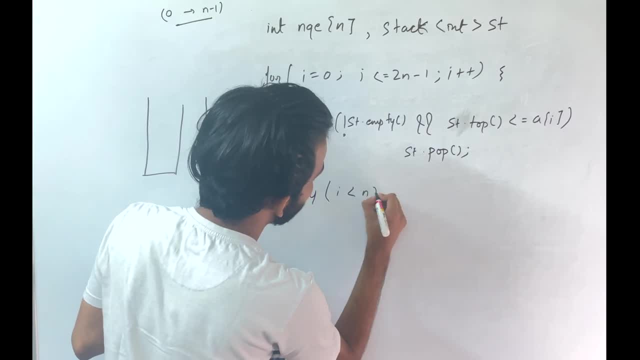 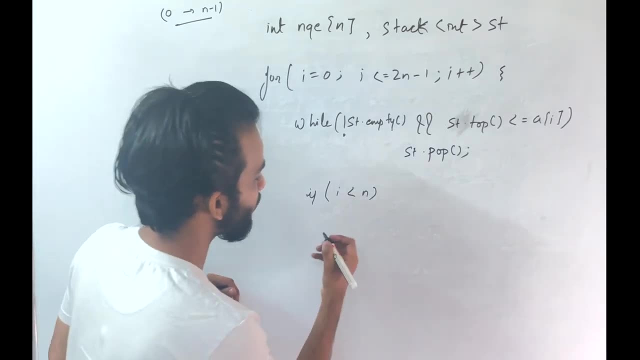 So what I'll say is: if, if x is lesser than n, then only I require the nge, because beyond, beyond the first half, I don't require the nge. So what I'll say is: if i is lesser than n. 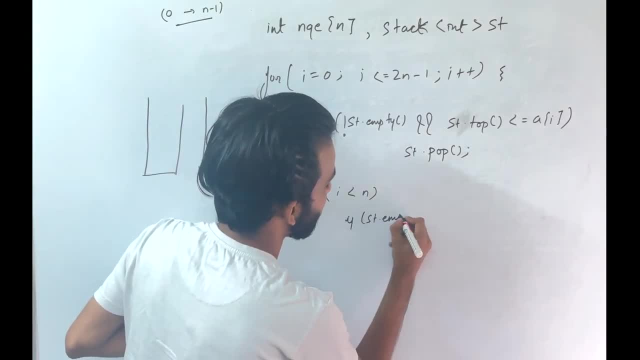 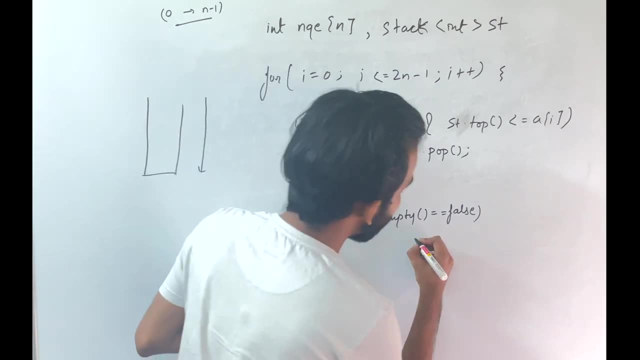 and if the stack is not empty? again, if the stack is not empty, then can I say, can I say my nge, yes, my nge of i is equal to stack dot top. If the stack is not empty. 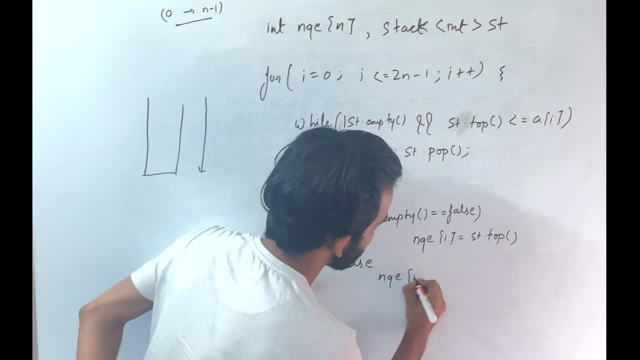 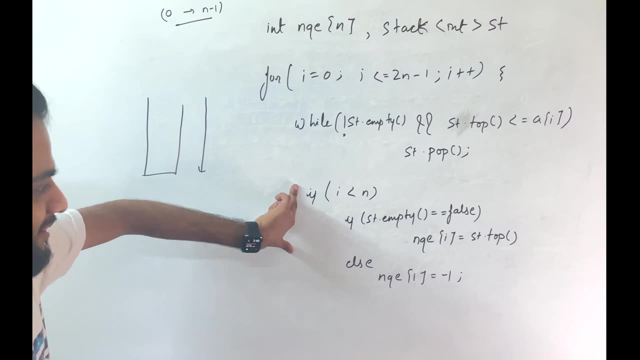 but if the stack is empty, can I say my nge is minus 1.. That's how you can definitely write. and what if this after this, what you have to take that element and you have to put it onto the stack. 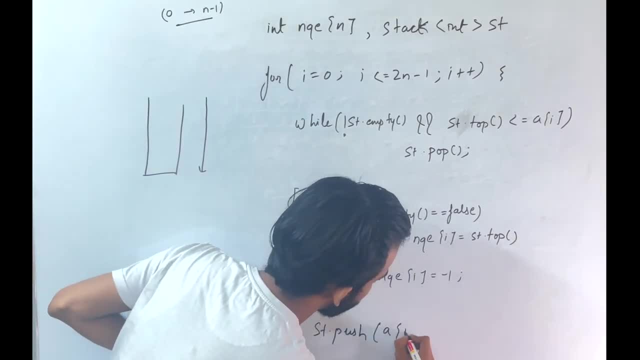 After that, please make sure you have to take that element and you have to put it onto the stack. So this is how your code for the first variant would have looked like, But I did tell you that everywhere. 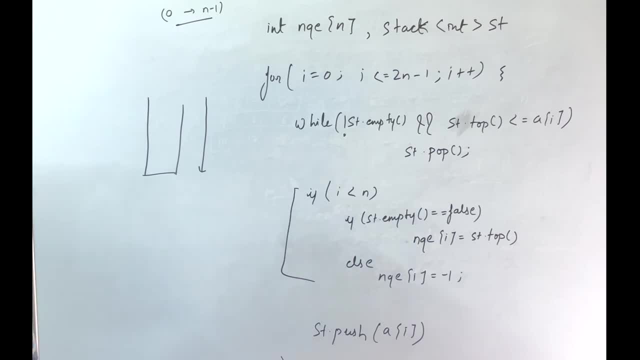 yes, everywhere. since you're implementing circular array, please make sure, instead of i you have to write i modulo n. Obviously over there and obviously over here. you have to write i modulo n So that you can directly access. 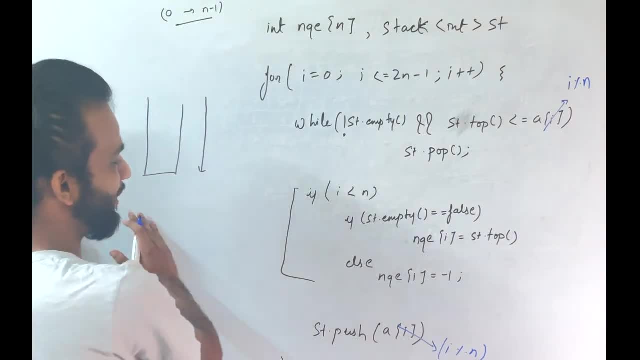 directly access the first half without actually making a copy of it. So this is how you can implement your nge. Now, what will be the time complexity of this one? I can say the time complexity. 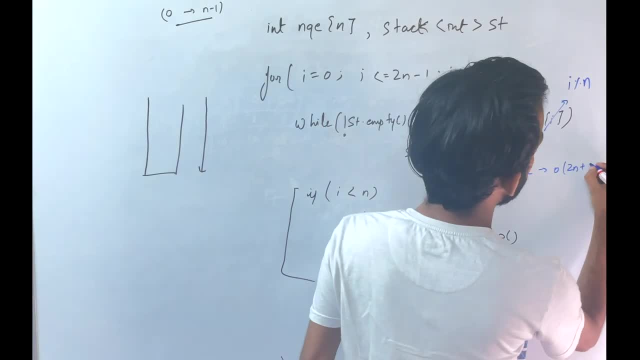 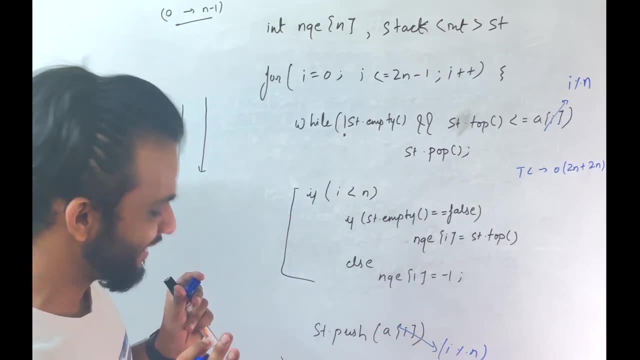 is a bigo of 2n plus a bigo of 2n. Now, why a bigo of 2n? Why not n square? Okay, Let let me just ask you a very simple question. This loop: 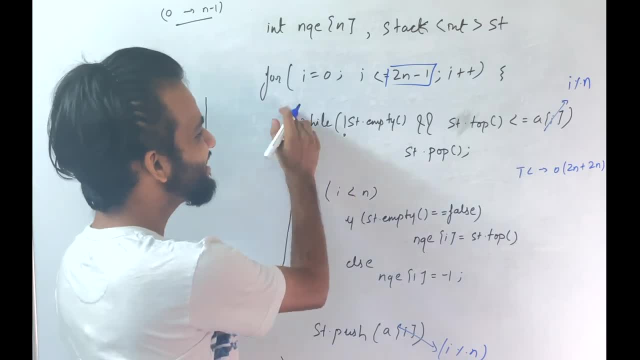 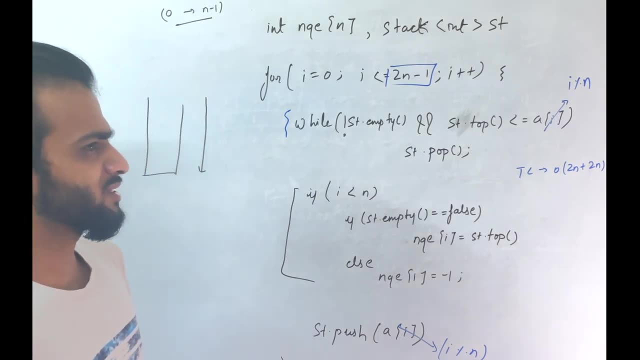 is running for 2n times. Everyone knows that. But is this loop running always for 2n times, Ask yourself, And the answer that will come is no, Because sometime this might run for one time might remove one small element. 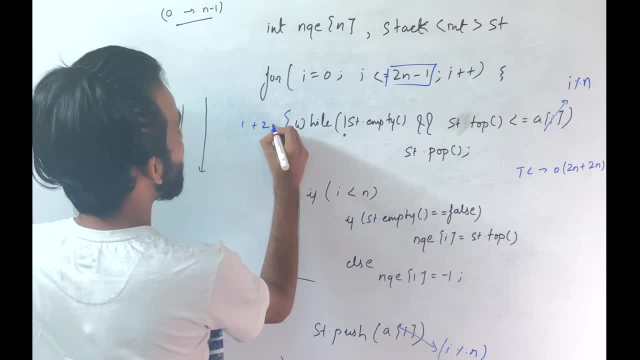 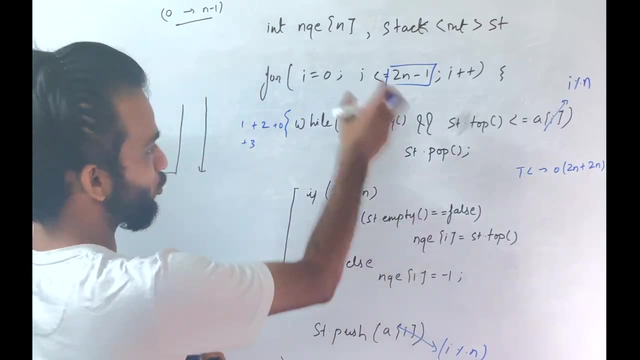 sometime it might run for 2 times. sometime it might run for 0 times. sometime it might run for 3 times Overall throughout throughout the iteration. like: how many times is this while loop executed? throughout the fall loop? 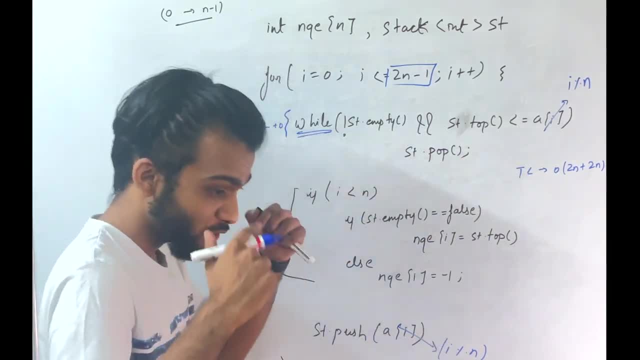 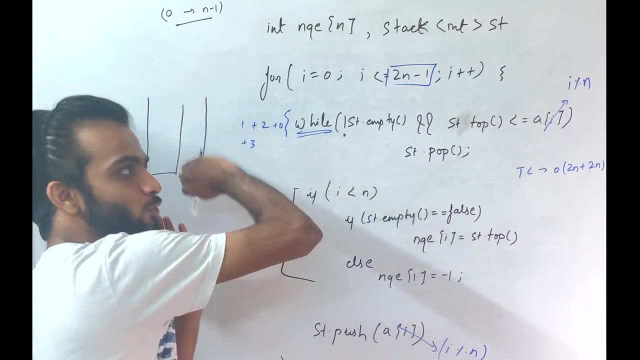 What will be the total number of iterations this while loop will be executed? If you think, won't it be the total number of elements of the array? Because those elements are getting in and those elements are getting out, Isn't it? 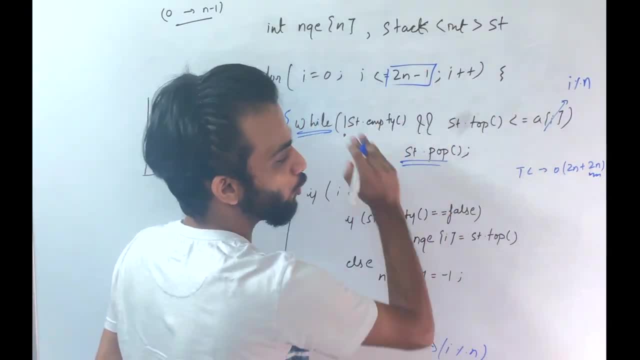 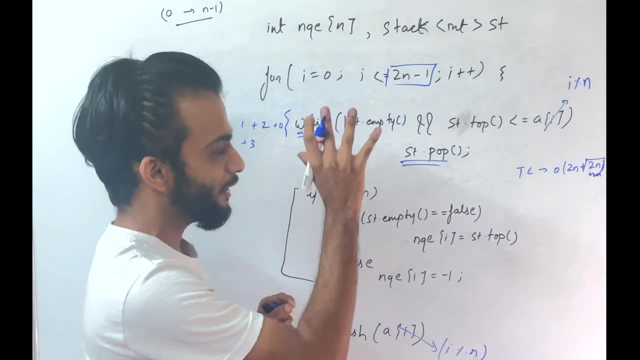 Hence the total iteration across the fall loop will be 2n of while loop. If you did not understand, I will just give you a very simple hint: While you code, just try to put a count plus plus.